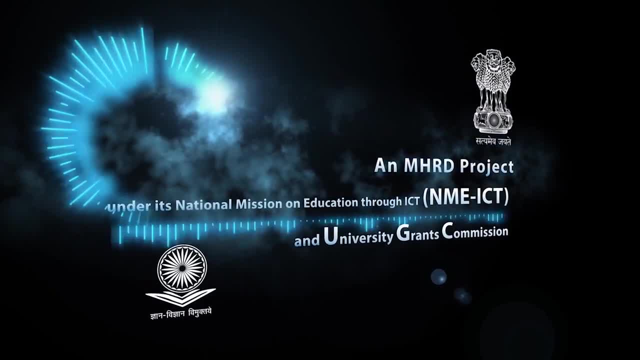 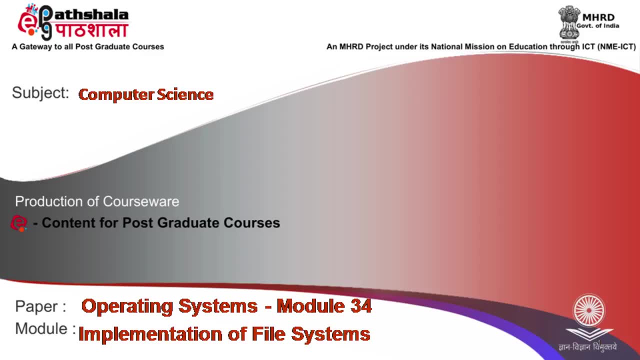 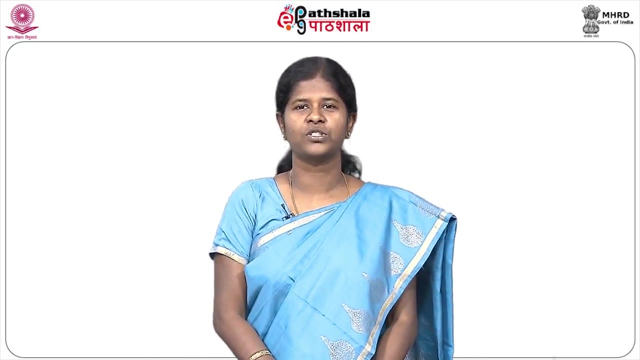 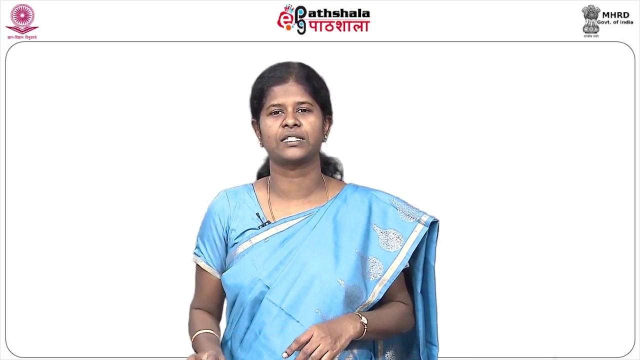 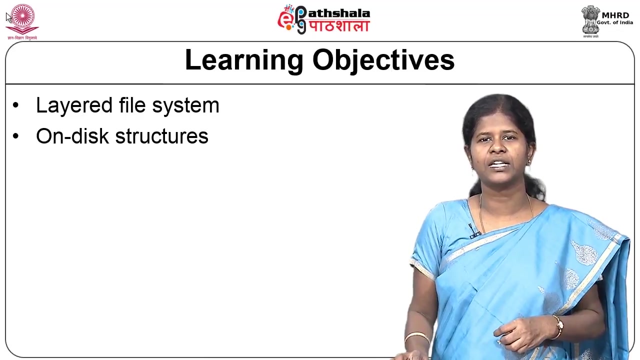 Welcome to APG Parsala lecture series in computer science. This course is on operating systems. In this module we will learn different issues related to implementation of file systems. The learning objectives for this module are to understand the different layers in a layered file system and, for the implementation of the file system, a number of on disk data. 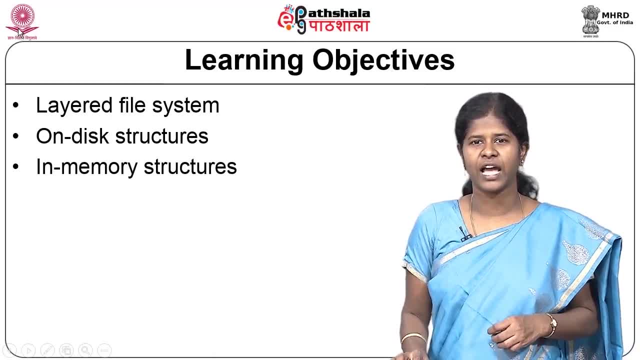 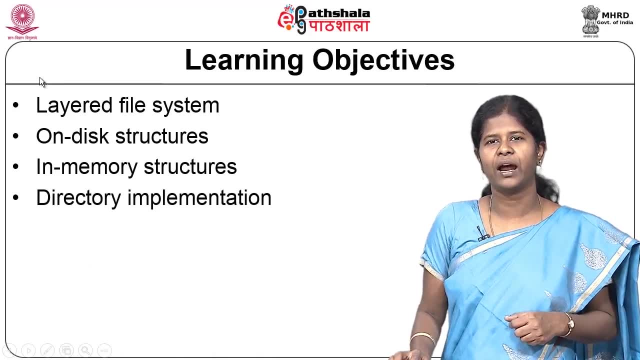 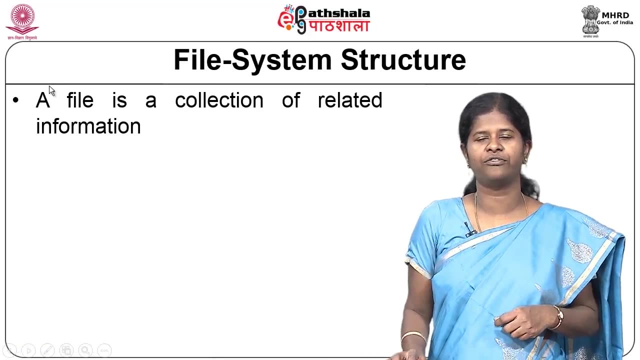 structures and a number of in memory data structures have to be used. So we will learn what are the different data structures that help in the implementation of file systems and we will understand how directories can be implemented. We all know that a file is a collection of related information. 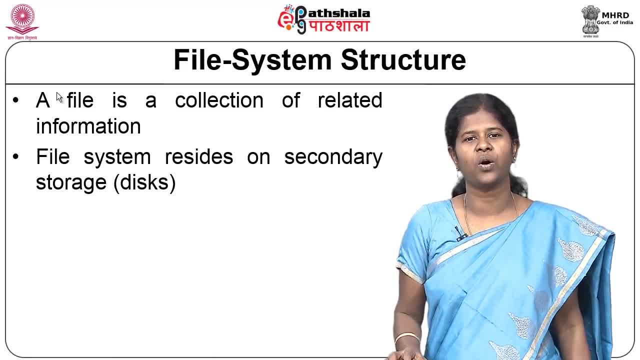 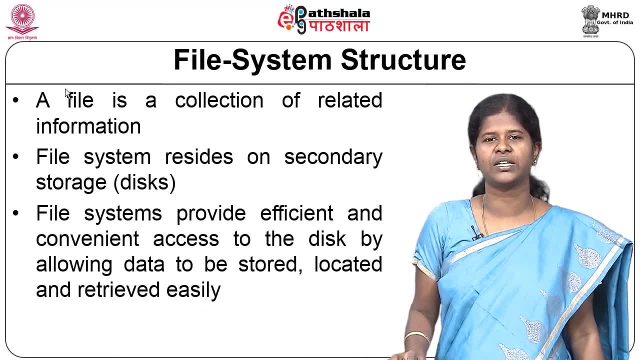 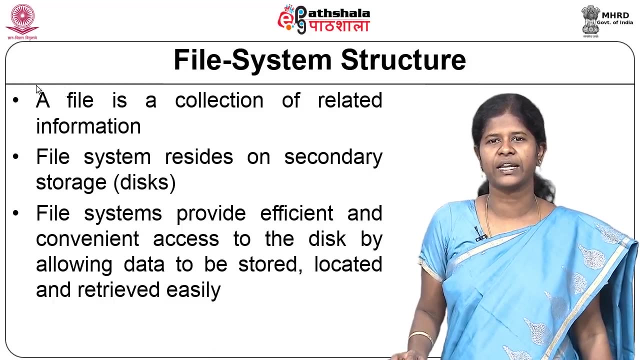 And file systems generally reside on secondary storage device or they are kept in disks, And this file system will provide efficient and convenient access to the disk by allowing our data to be stored, located and retrieved easily from the disk. So if there is no proper 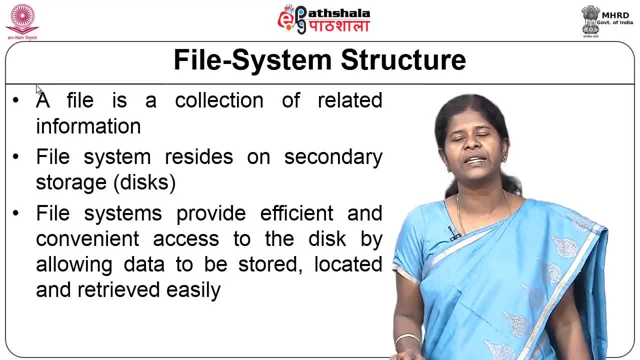 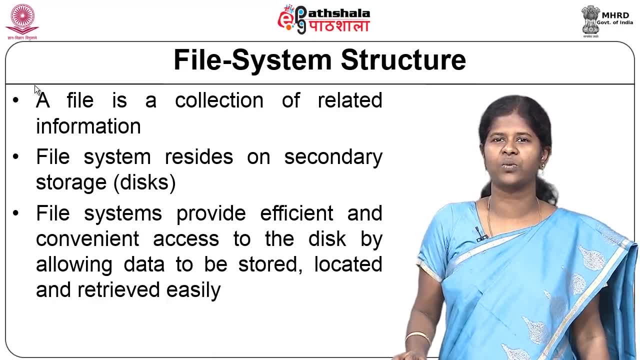 structure. when you are placing information in the disk, then in that case, like it will be very difficult to know to retrieve data from the disk, to know where the data is kept in the disk and so on. So, rather than randomly placing information in the secondary storage, 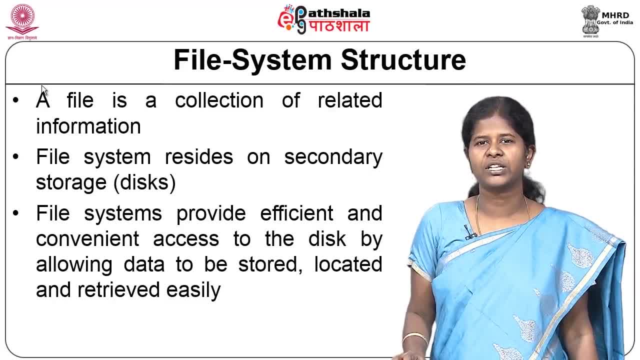 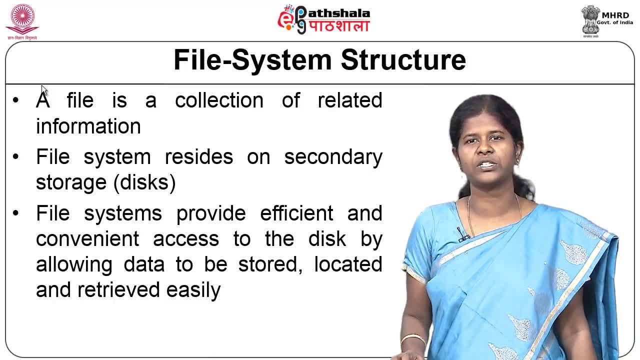 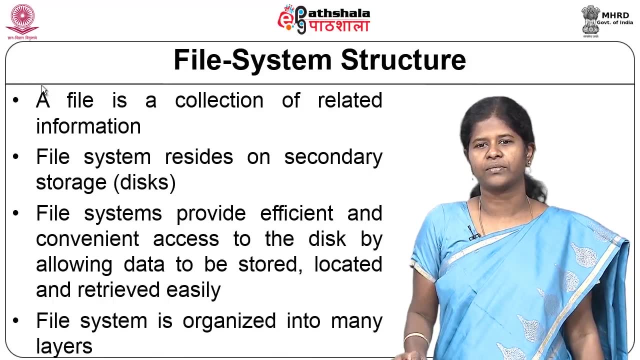 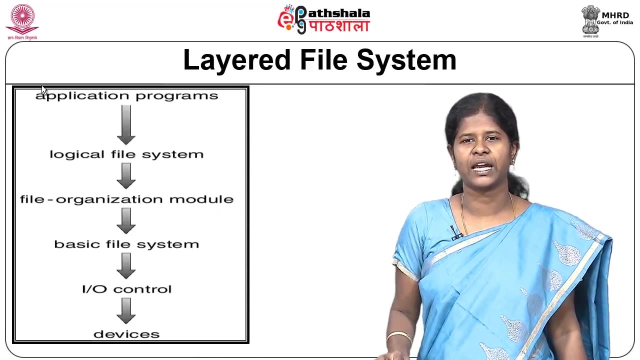 device or in the disk. you structure in terms of files and the files can be kept beneath directories And you have a file system kind of a structure, a proper structure, and use that structure for easily retrieving and placing information in the disk. So the file system is generally organized into many layers. We see the different layers. 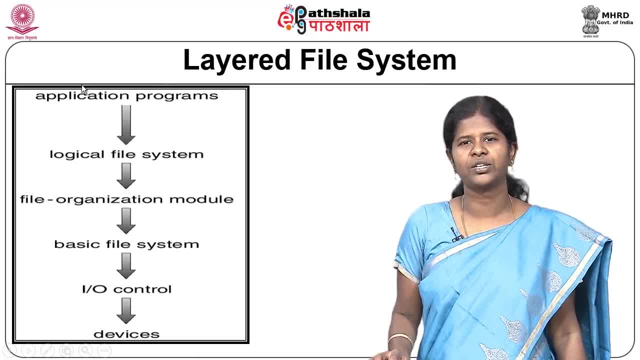 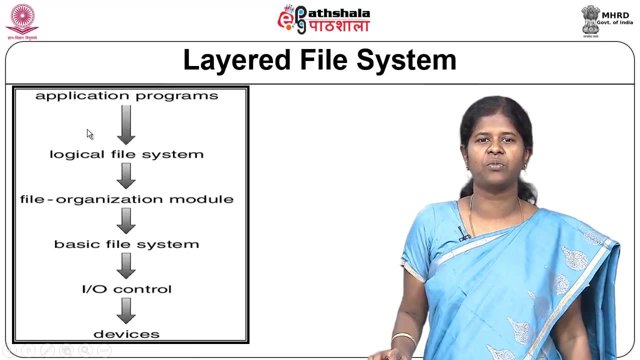 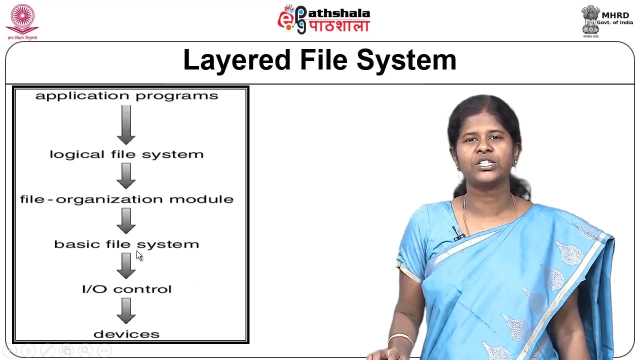 are kept in a file system. You have the application programs returned by the users and the users application programs will use the logical file system and the logical file system will invoke different data structures and modules in the file organization module. and the file organization module will use a basic file system which in turn will use the I O control. 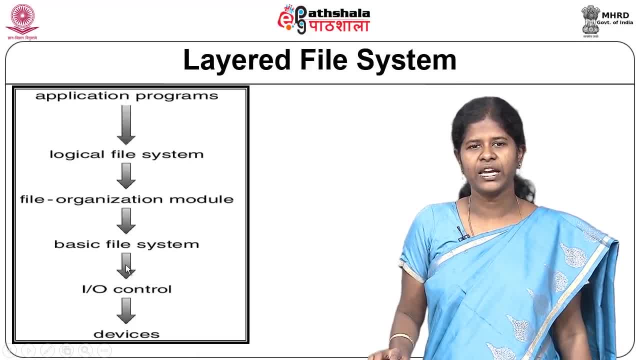 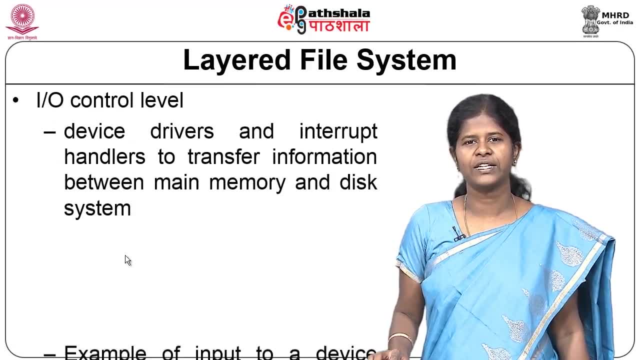 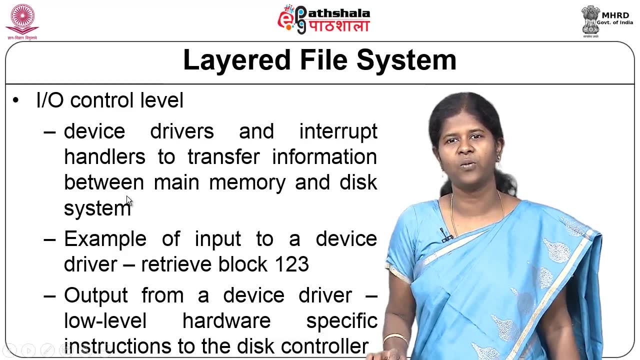 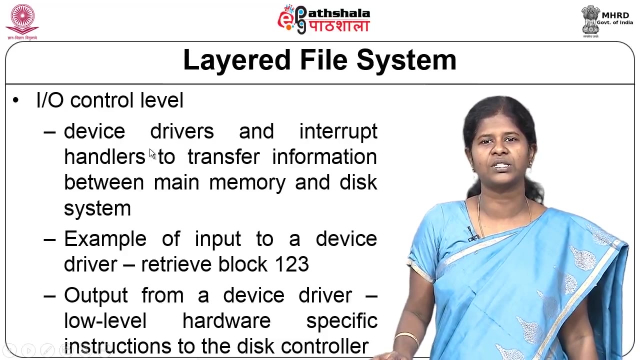 which in turn, will access the I O devices. Now we will see each of these layers and the functionalities of each of these layers. So first we will look at this I O control level and the I O control layer which is placed just above the devices. So what go into this I O control level? Those are the device drivers. 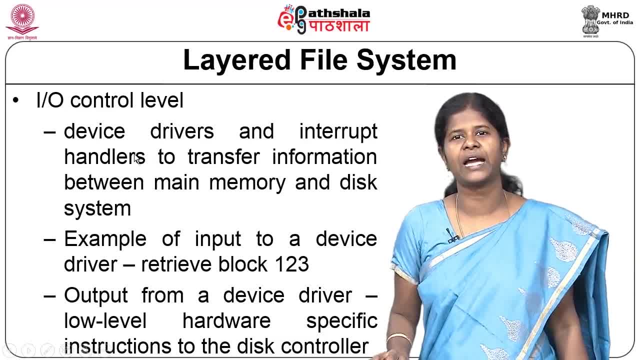 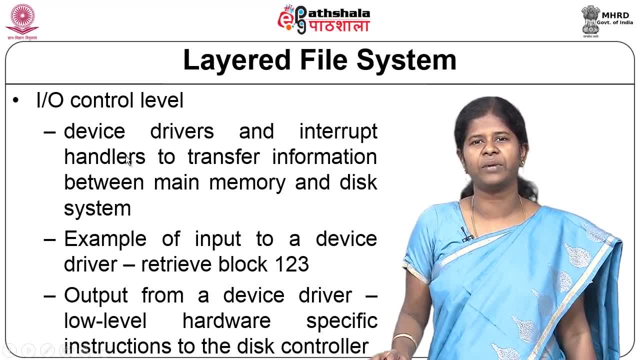 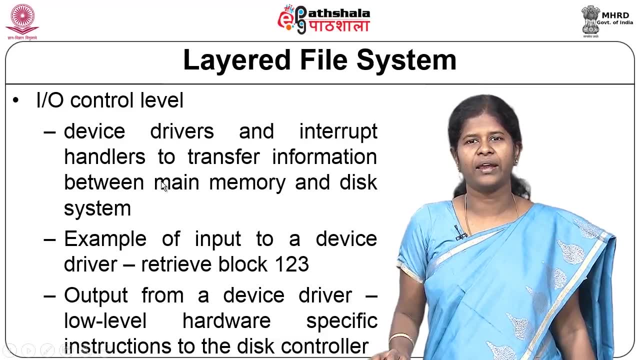 and interrupt handlers. So device drivers actually act as an interface between devices and the operating system. They help to transfer the information between the disk or the device and the main memory. So an example of input that is given to a device driver will look: 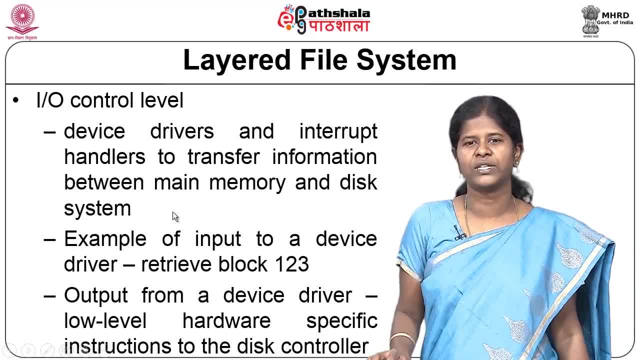 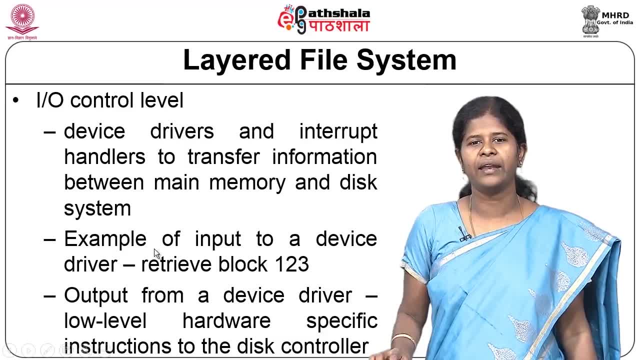 something like retrieve block number, block number 123, from the disk, And when this instruction is given to the device driver from the upper layer, then the device driver will have to produce the I O control layer. So this is the I O control layer which is placed just. 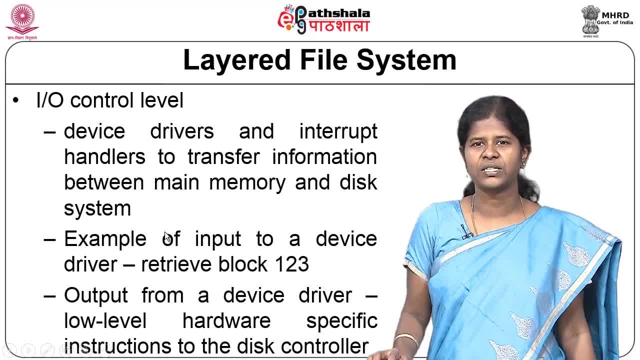 above the devices and the operating system. They help to transfer the information between the devices and the main memory, And when this instruction is given to the device driver from the upper layer, then the device driver will have to produce low level hardware. specific instructions to the disk controller, And the disk controller will help assist in reading. 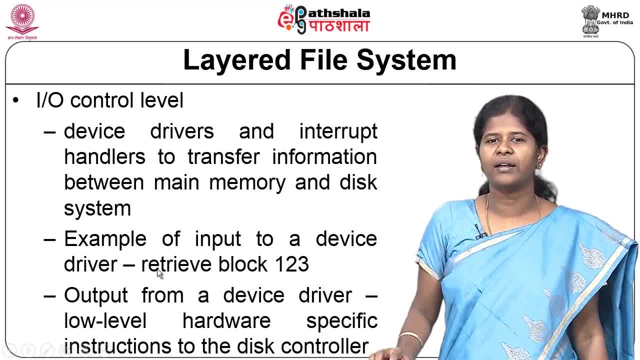 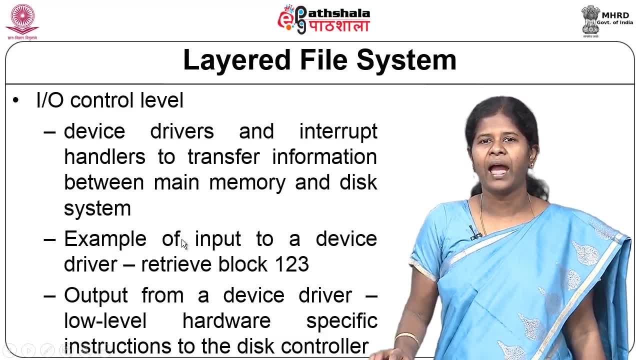 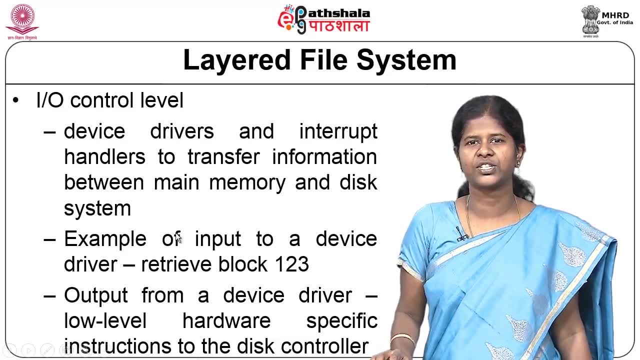 and writing from the disk. So basically, here you have an instruction called retrieve block, which means you need to read the contents of block number 123.. And the device driver will know how to translate this into hardware specific instructions and it will provide instructions to the disk controller which in turn will take care of reading from this block number. 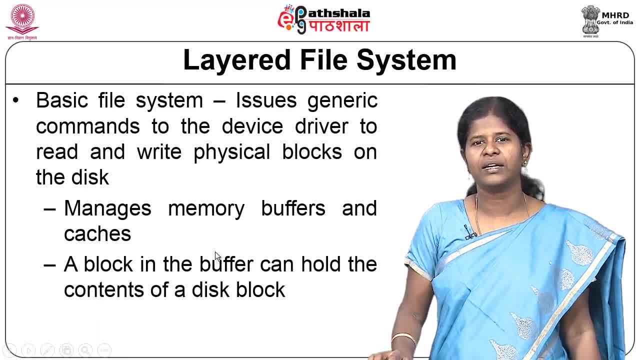 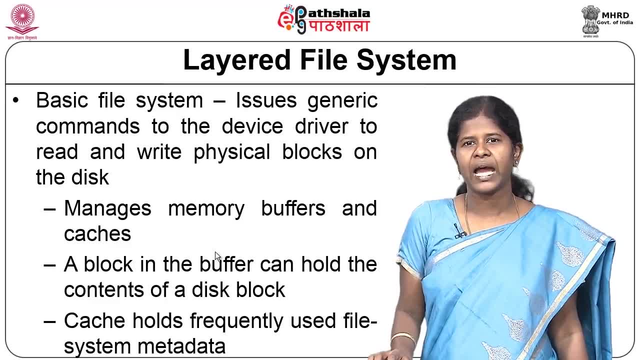 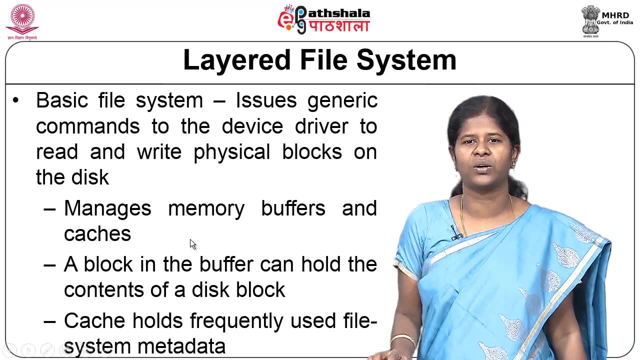 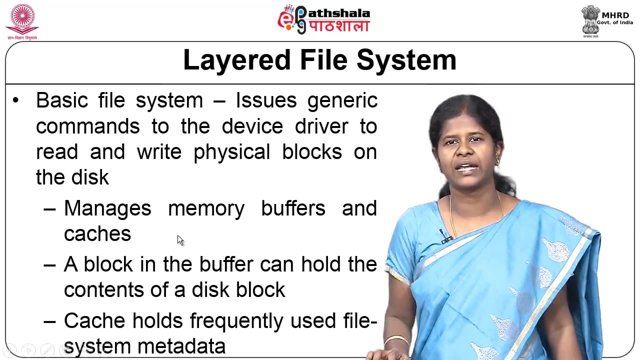 123. And the next level is the basic file system. This layer sits just above the I O control and this will issue generic commands to the device driver to read and write physical blocks on the disk. This also manages memory buffers and caches. So memory buffers and caches are 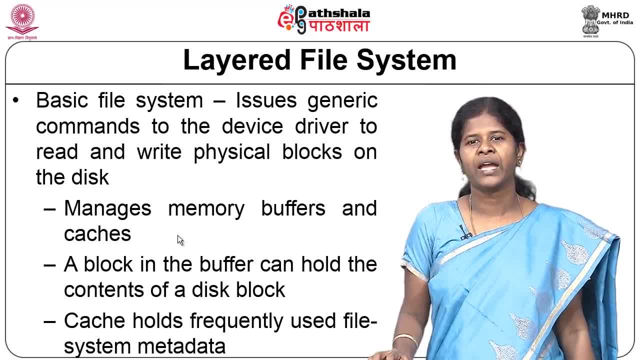 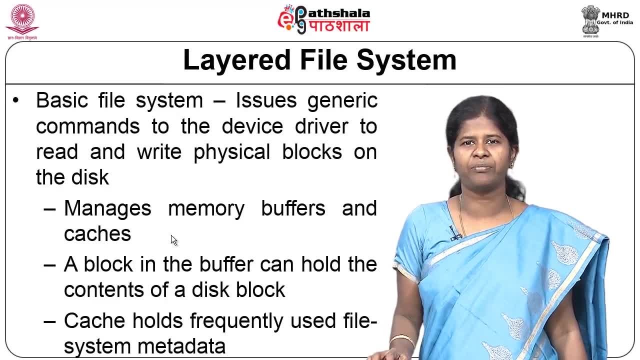 maintained by the operating system in the main memory, And a block in the buffer can hold the contents of a disk block. So you have a number of memory buffers that have been maintained may be. it is called the buffer cache And each buffer in this buffer cache 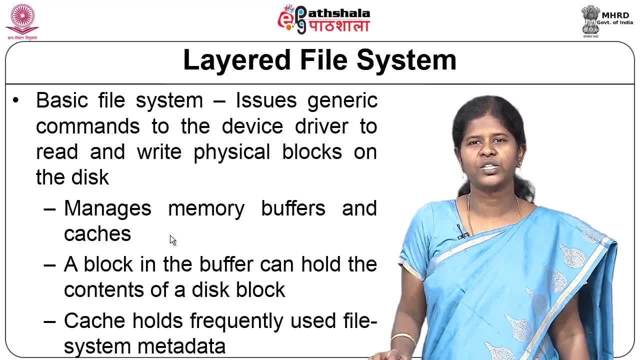 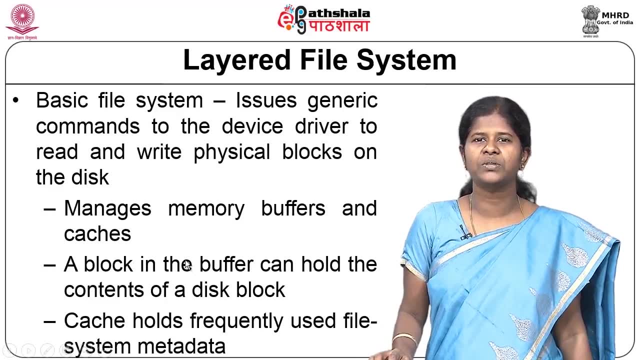 can hold a blocks data. So whichever is read from the disk is copied on to these buffers in the buffer cache And they can be used later if there is a hit or hit again, And you also maintain cache, a cache which holds frequently used file systems. 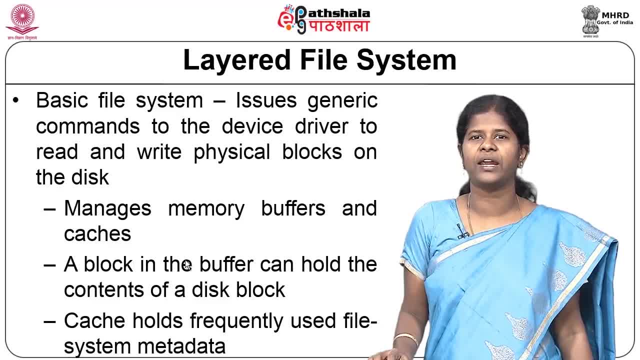 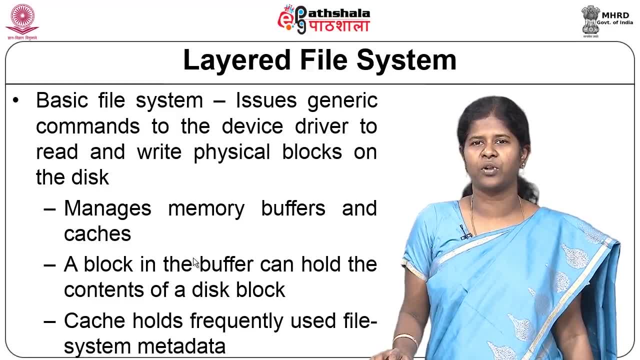 metadata. It can even be the contents of a file, or it can even be information related to the file, like the owner of the file, size of the file or the file control block, etcetera, and so on. So metadata related to the file can be cached And if the file is being used. 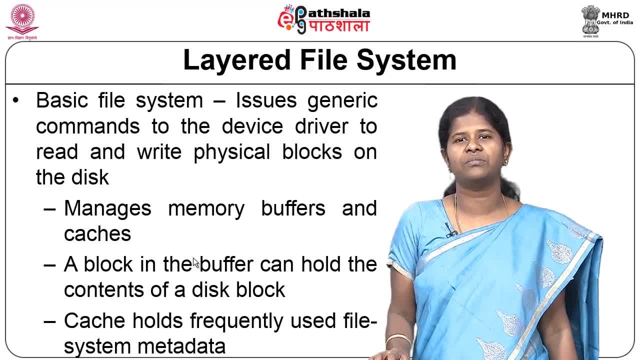 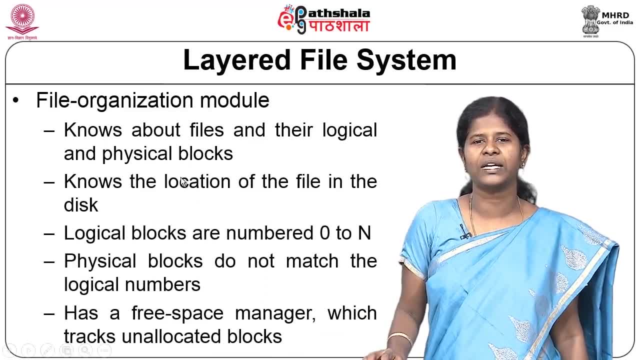 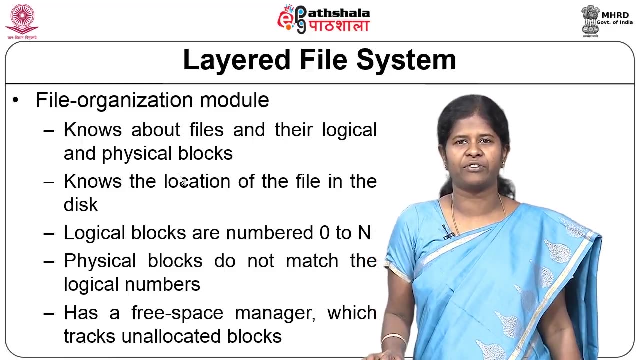 very frequently. then that information can be got from this cache itself. And now we have this file organization module. This, it is about this basic file system. This file organization module knows about the files and their logical and physical blocks. Logical blocks are with respect to a particular file. For each file, the logical block number will 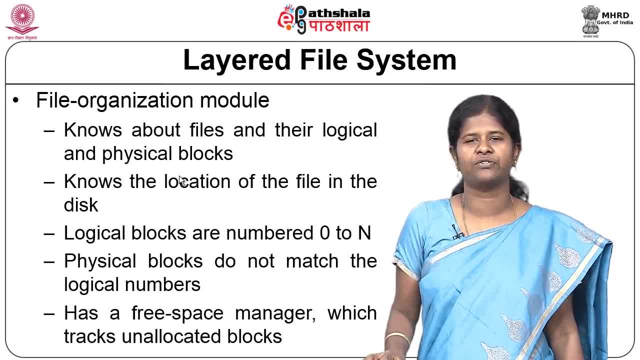 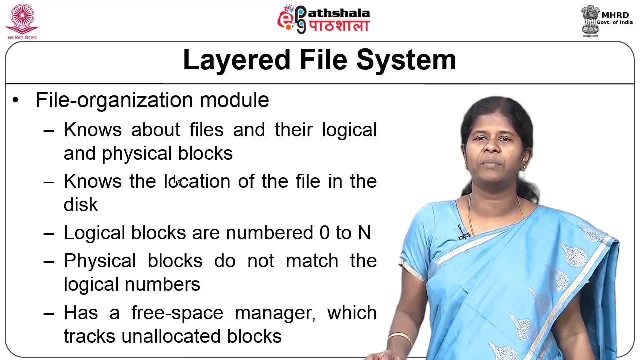 go from 0 to some n depending on the size of that particular file. But these logical block number or if it is first block in the file, that need not be mapped on to block number 1 in the disk. it can be kept anywhere in the disk. So the physical block number will be different from the logical. 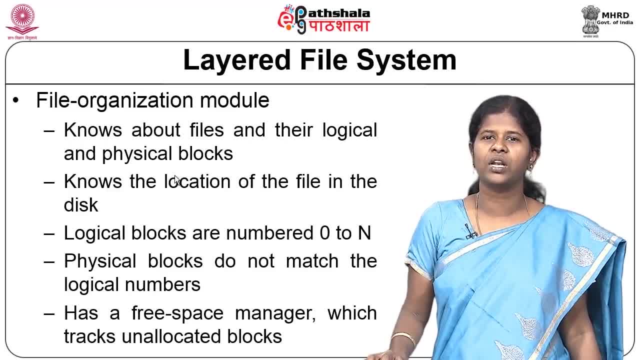 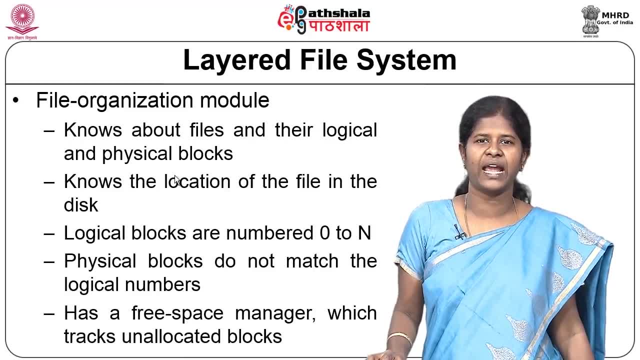 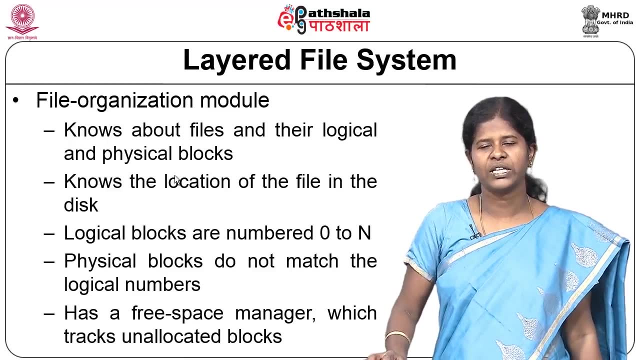 block number, So the physical blocks need not match the logical block number. So it is necessary to know where block number 1 of, say, file x is kept in the disk, or it is necessary to know the location of the file in the disk. So for this appropriate data 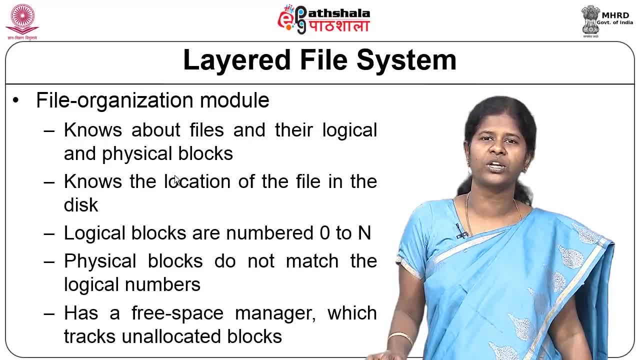 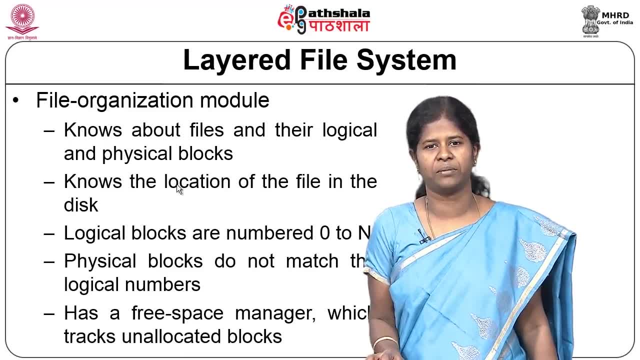 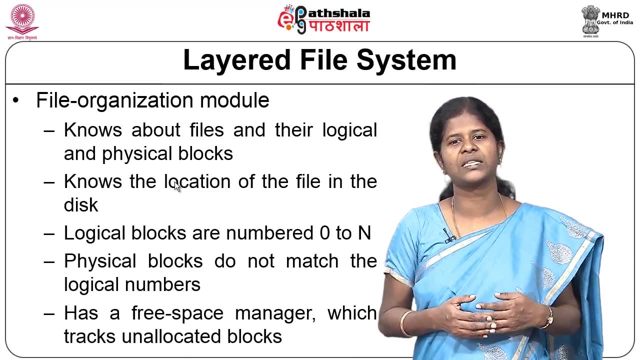 structures and information is maintained by this file organization module to know the mapping between the logical block number of the file and the actual physical disk block number, The file organization module. it also has a free space manager which tracks unallocated blocks. So in the disk you have a number of disk blocks or the disk is divided into. 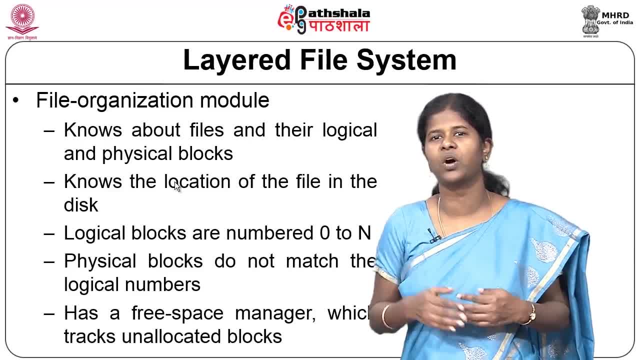 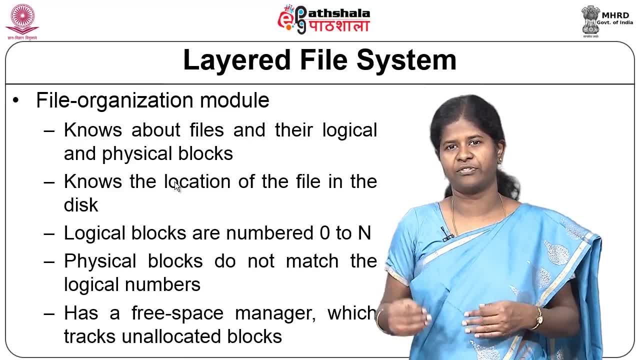 a number of disk blocks and file contents are placed in the disk blocks in the disk and some blocks will be allocated, which holds the contents of the file, but there will be some blocks which are not allocated, which are free for use. So the file organization. 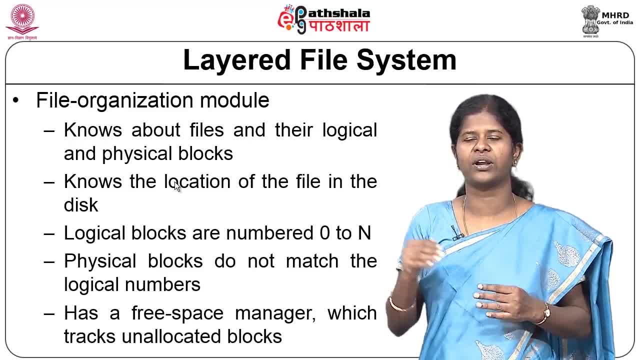 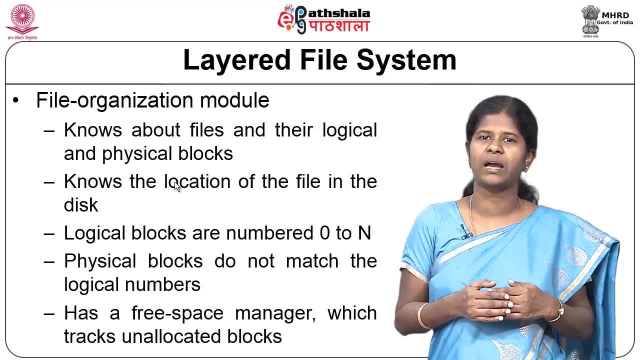 module maintains information about which blocks are allocated and which blocks are free. So if you know, if it knows the free blocks, then the next time a request comes to store the contents of a file it will know. these are the blocks that are free and those blocks. 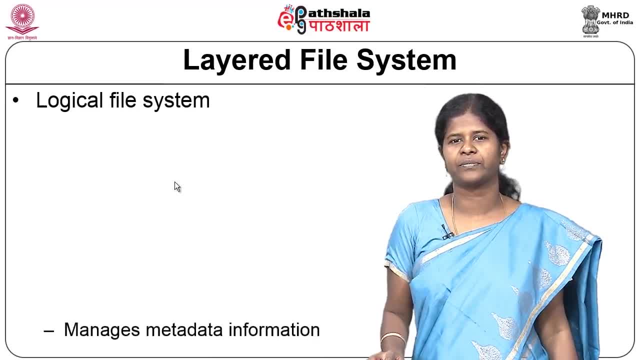 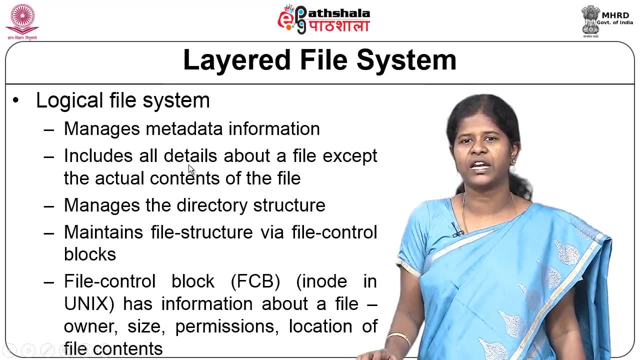 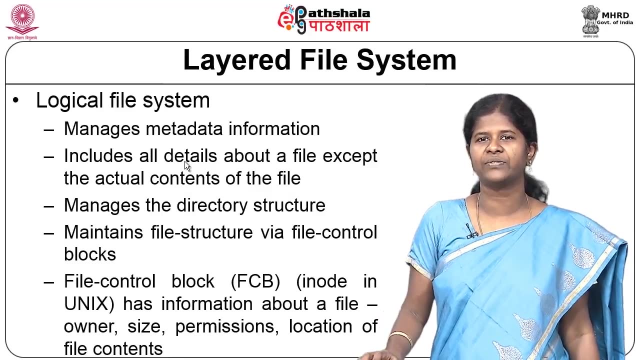 can be used for storing the contents of a file And then about this layer. you have this logical file system. This manages the metadata information about a file, or it will have all the details about the file except the contents of the file. The contents of the file will be kept in the disk, but all of the information of 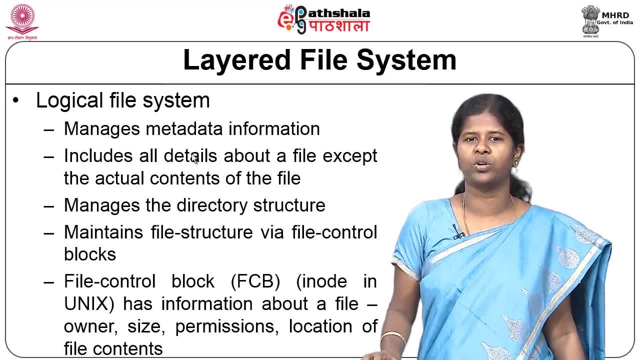 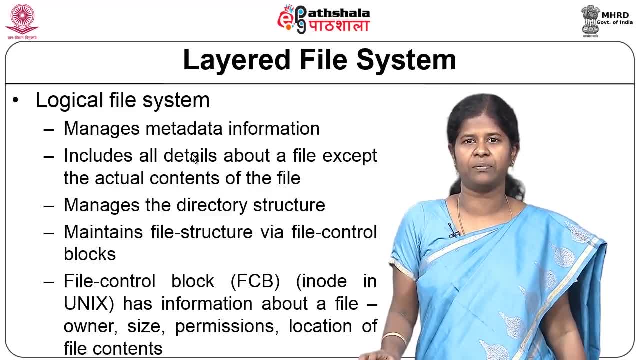 the file, like the size of the file. the owner of the file permissions- access permissions of that file. it will know the locations of the disk blocks where the contents are kept. the actual contents will not be maintained, But the name of the disk blocks, the number of the disk blocks where the actual contents 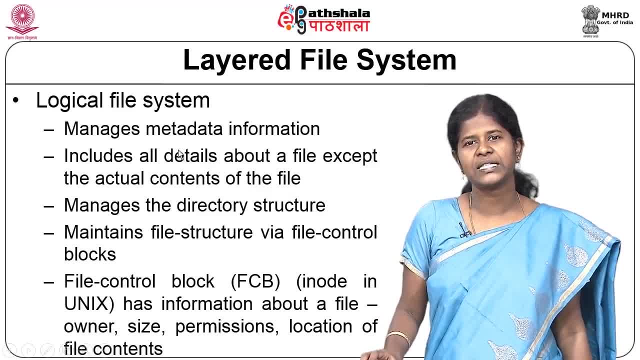 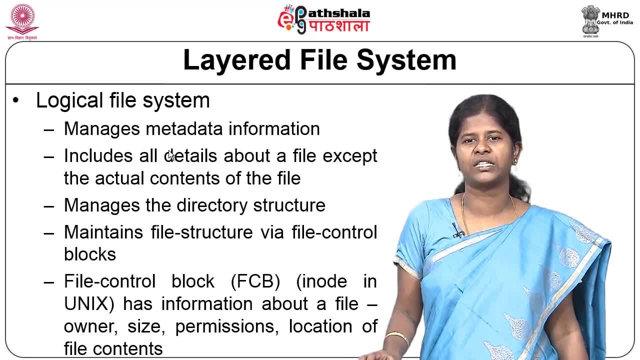 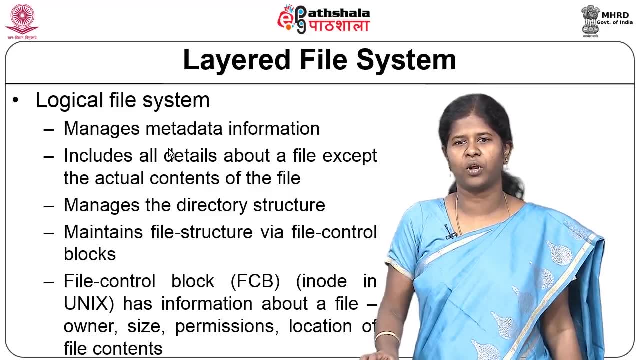 are kept will be maintained. Then it maintains the directory structure that is in this particular directory, which are all the files that are kept. that kind of a directory structure is maintained and it will maintain information about the files, which is called the file structure, through a file control block, And this file control block will have all this metadata. 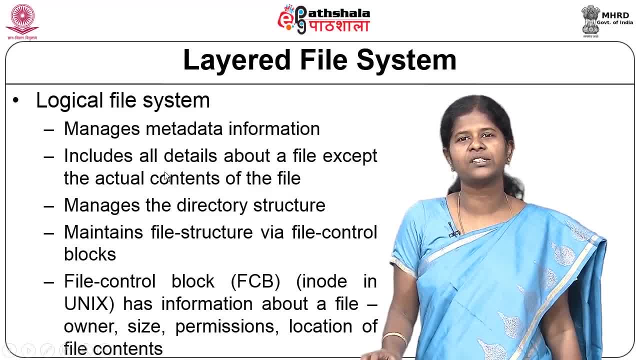 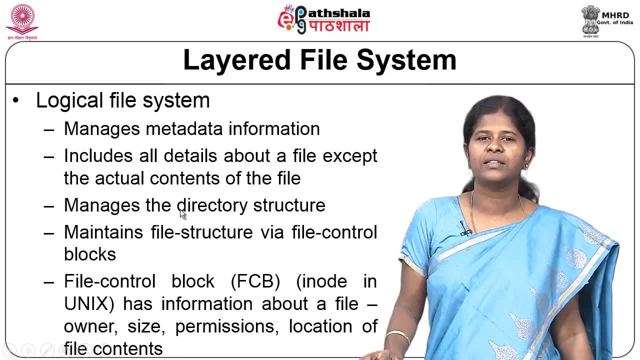 information. So this file control block, it is called the, an inode in unix. It has got information about a file, like the owner of the file, size of the file, the time when it was last accessed, when it was modified, the access permissions. 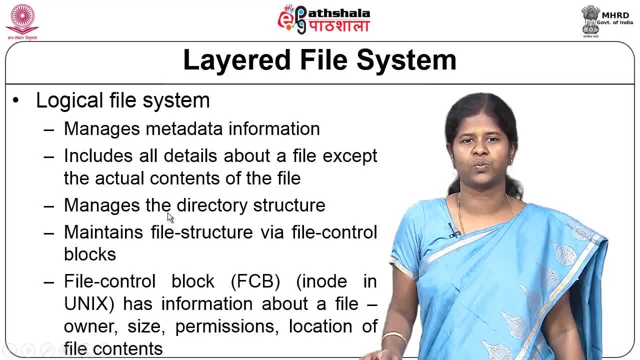 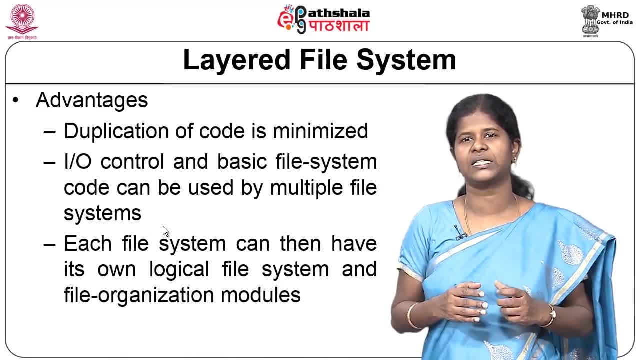 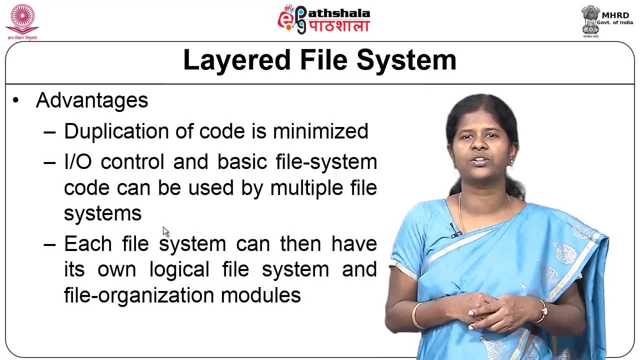 for the file, the location of the files, contents and so on. So we have seen that the file system is not maintained as a single layer, it is maintained as a multiple layers. So because of this, the advantages are that the duplication of 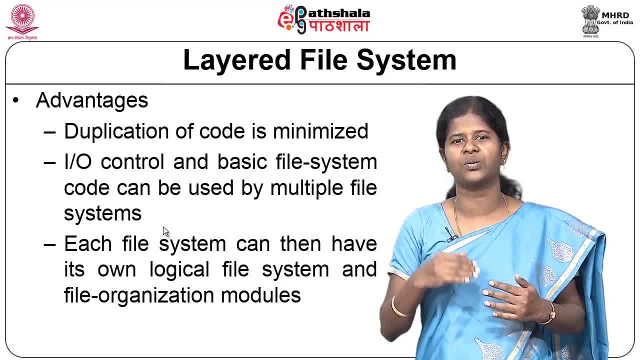 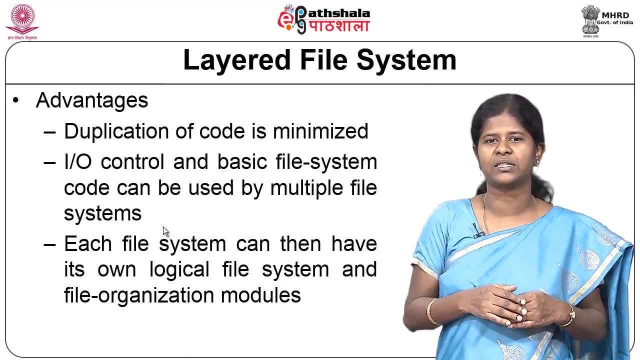 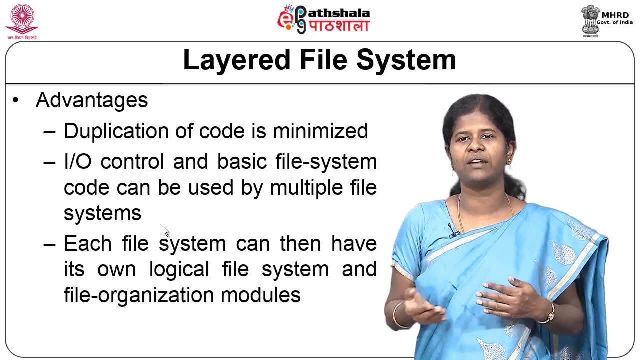 code is minimized And the lower layers, the IBO control and the basic file system code, can be the same for different file systems And above that, the other layers above that can be modified for each different file system or each file system can have its own logical 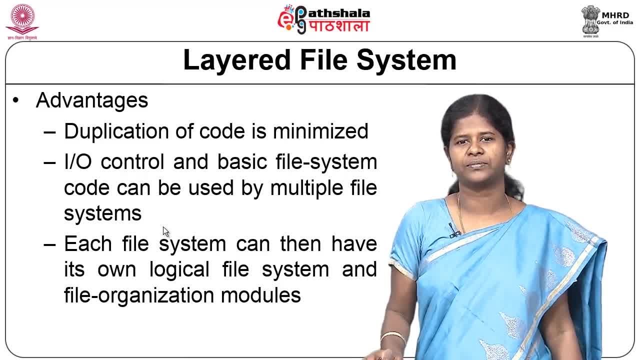 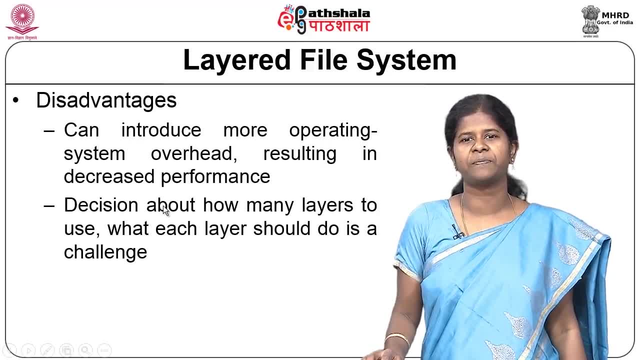 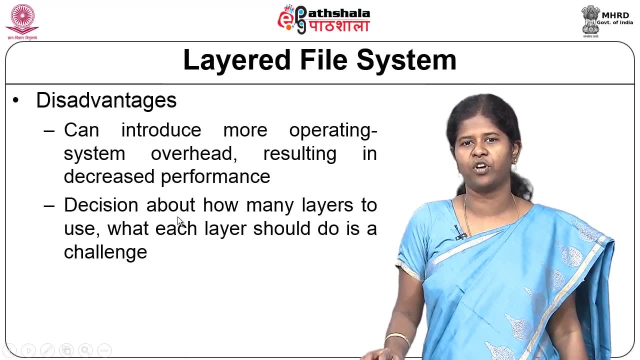 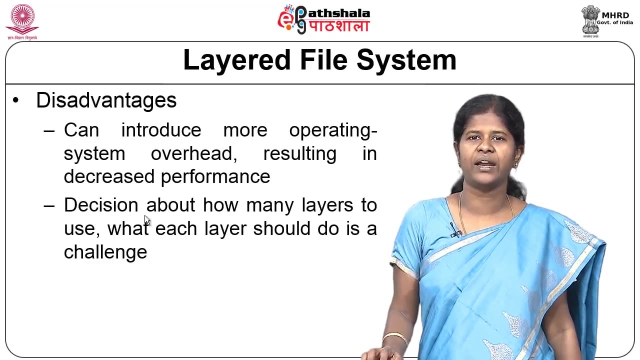 file system and file organization modules. But the disadvantages of this layered file system is that it can introduce More operating system overhead and because of that it can result in a decreased performance. And when the design of this layered file system is being done, it is necessary to decide how. 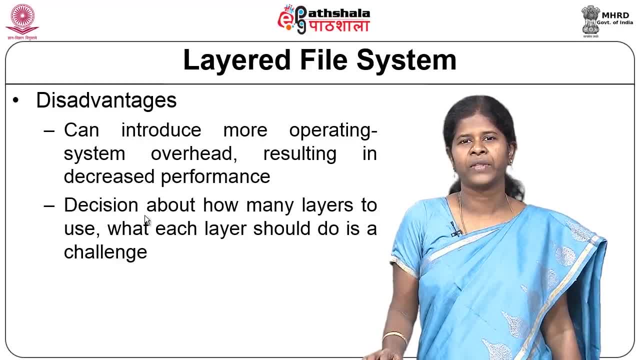 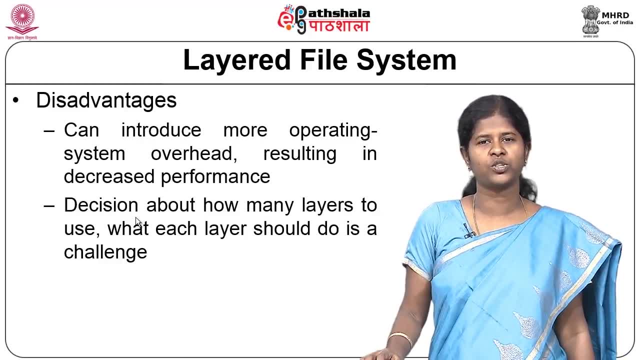 many layers you are going to use for the file system And what each layer should do, and each layer should have a different job both. there should not be an overlap in the working in the different layers, And this becomes a challenge when a file system 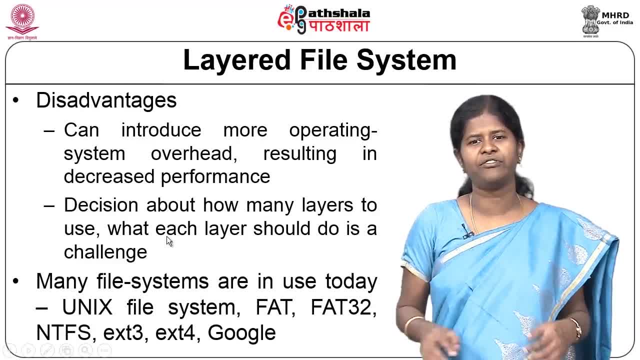 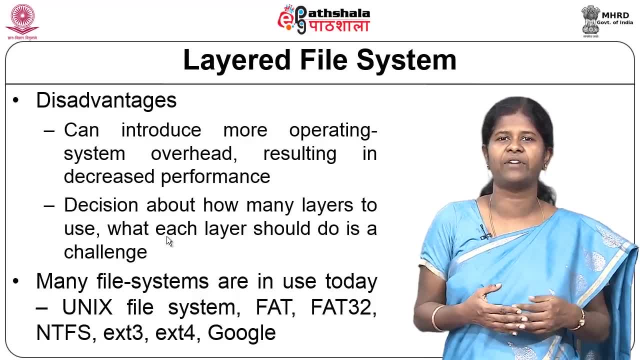 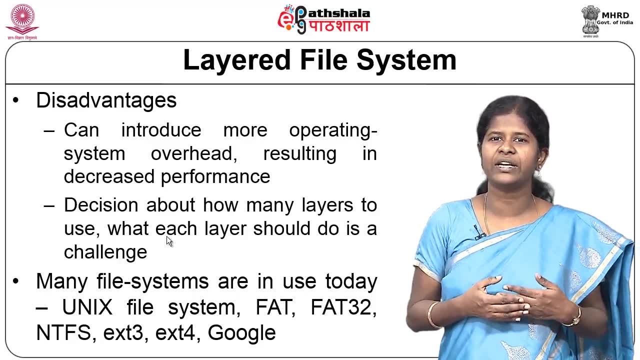 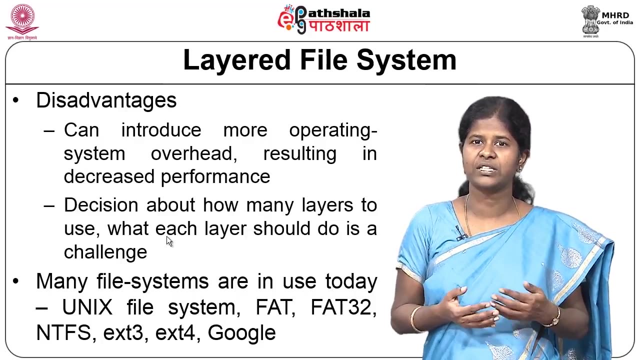 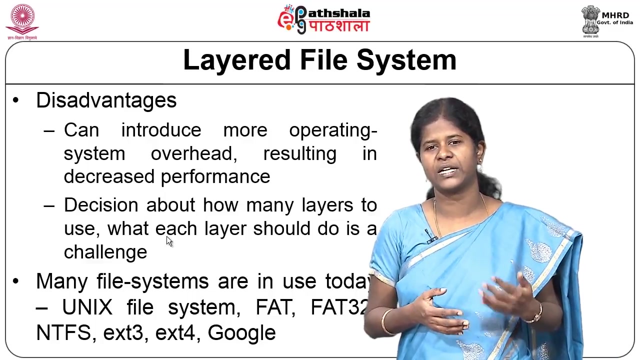 or a layered file system is designed, So there are many file systems are used today, like the Unix file system, the FAT, FAT32, NTFS, CORLF, egy flavors that are used in the Linux file system, and Google has developed its own file system. 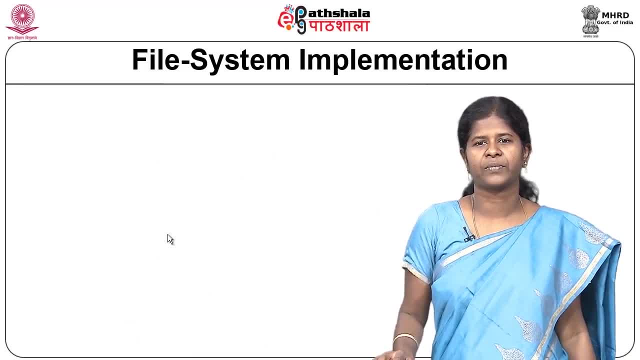 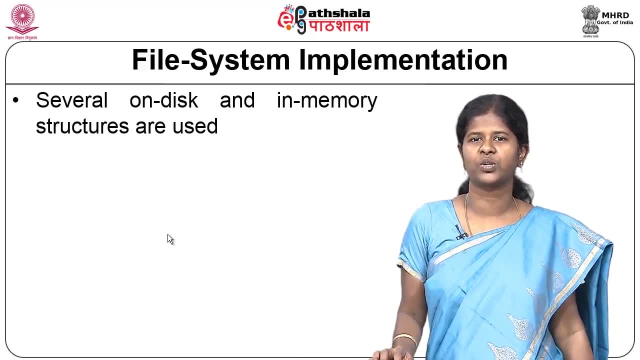 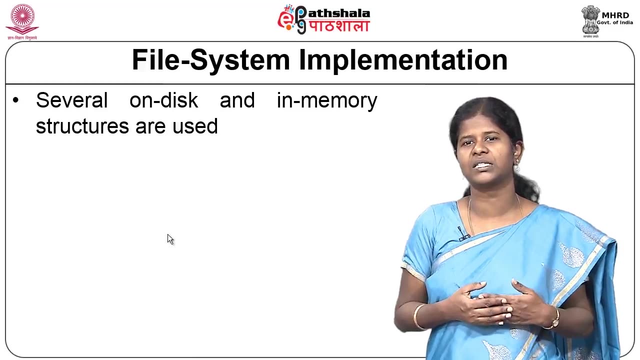 for its use, which is called the Google's file system, And now we will learn different issues related to the implementation of a file system. We saw that a file system can be layered, but now we will now learn different data structures that are being used to assist the implementation of the file system. 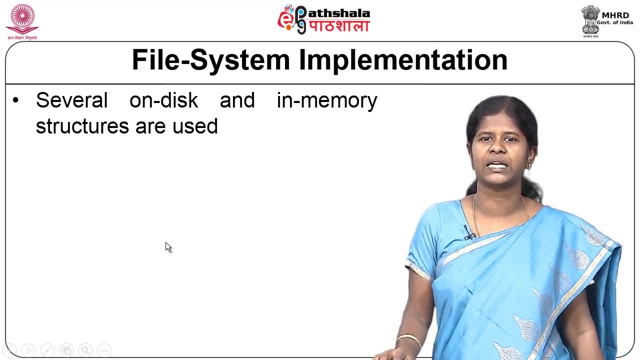 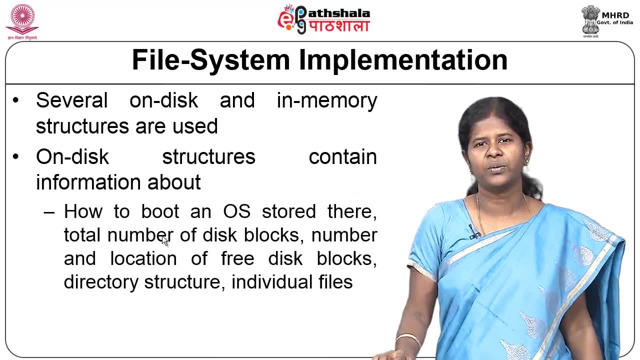 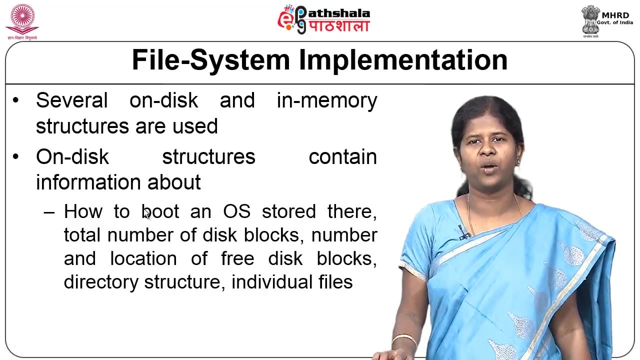 For a number of structures are being kept on the disk as well as in the main memory for the proper operating operation of a file system. So in the disk, structures are maintained which will have information about how to boot an operating system that is stored in the 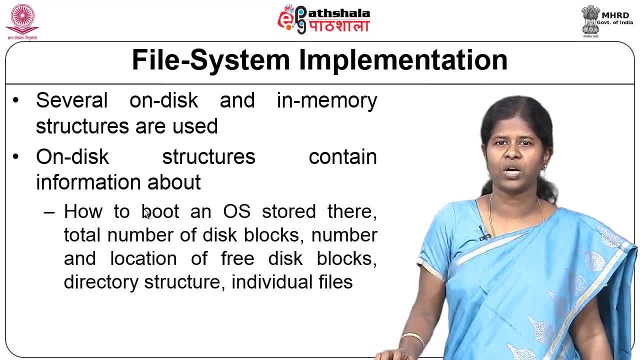 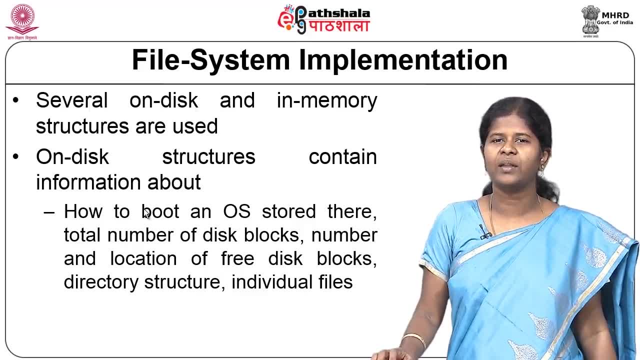 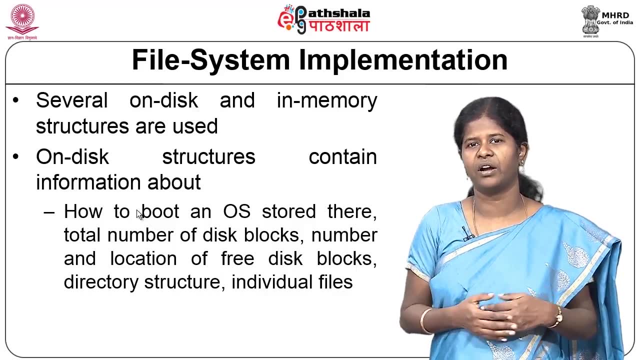 disk and the total number of disk blocks that are present in the disk and of these total number of disk blocks, how many are free disk blocks And which is the location of the disk blocks which are free? and what is the structure of a directory, what is the contents of each directory and individual files? So information. 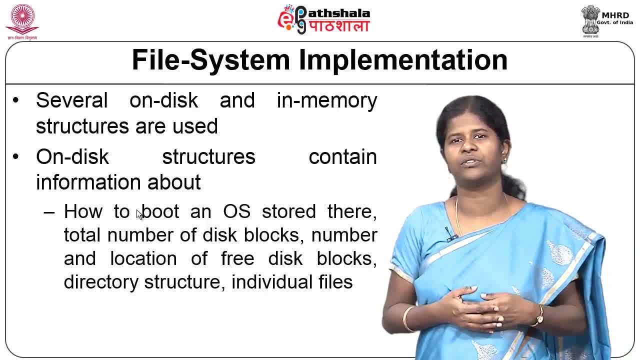 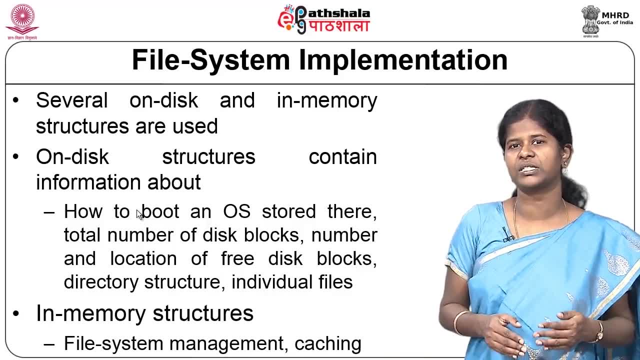 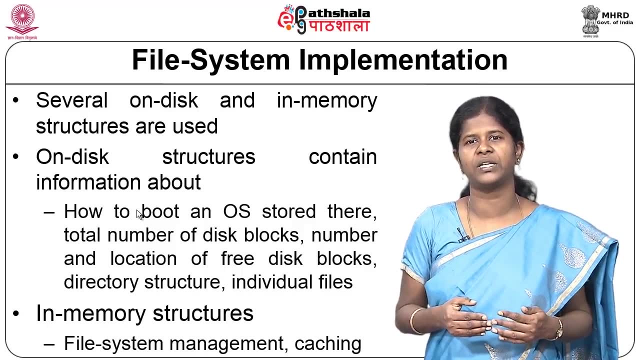 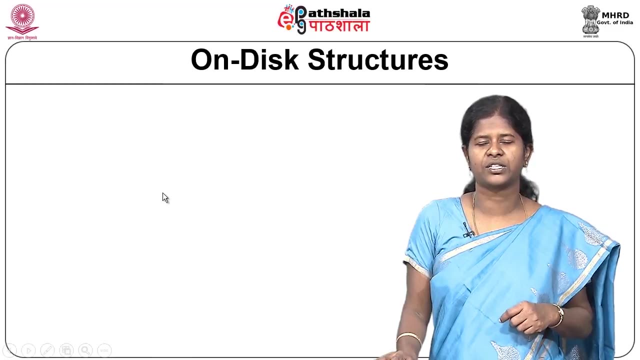 about individual files, say the inode in the case of Unix. all these are maintained in the disk And you also have a number of in memory structures and these structures are maintained in the main memory and these are helpful for file system management, For caching and so on. So now we will see each of these on disk data structures First. 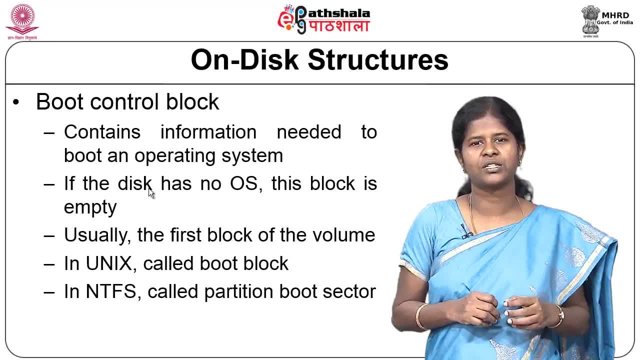 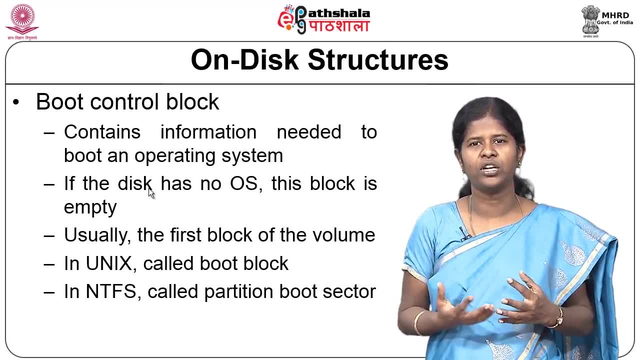 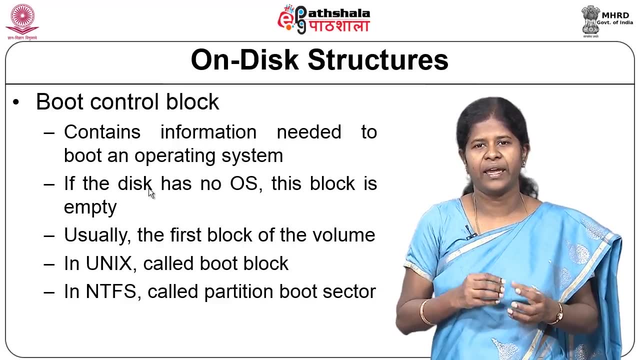 is a boot control block. This boot control block is usually the first block that is kept in the disk. Say, if the volume of the disk or a partition of the disk has an operating system or stores and operating system, then information about how to load the operating. 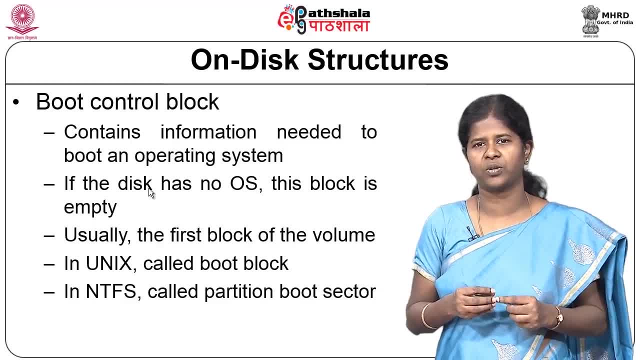 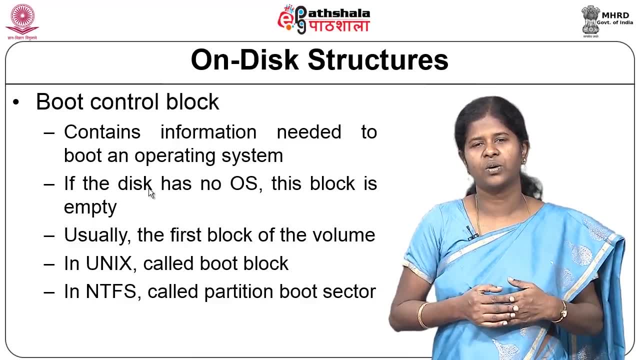 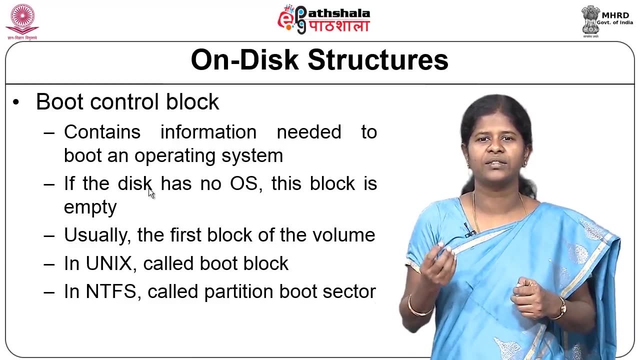 system into the main memory is maintained in this boot control block. We all know that an operating system has to be loaded into the main memory while the system works. So at the time of boot up, the boot stop load up will try to find out this sector 0 or the. 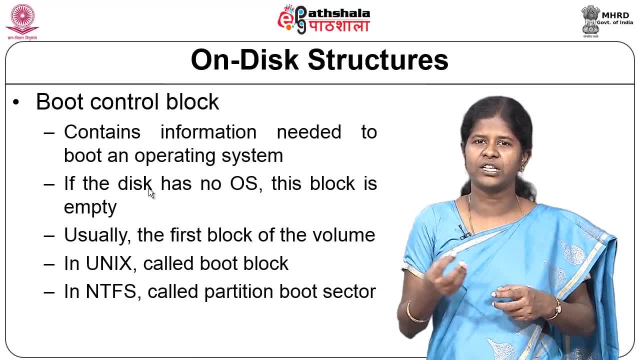 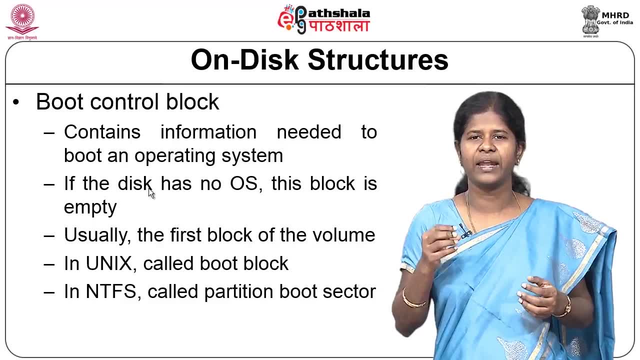 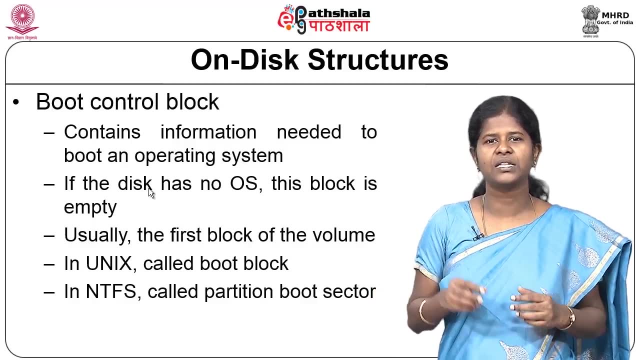 first block present in that partition and you the partition will have information needed to boot the operating system. Suppose, if that partition does not have an operating system, then this block will be empty. the boot control block or the first block will be empty. In UNIX this boot control block is called a boot block. In NTFS operating system it 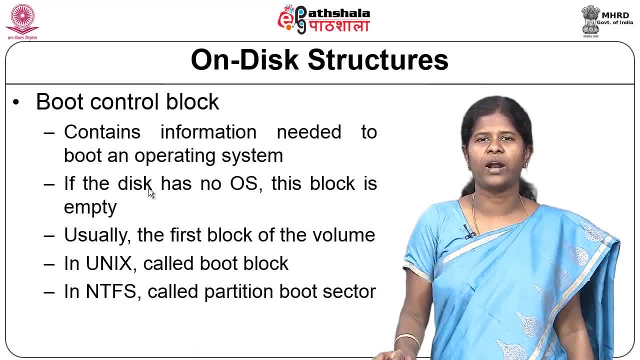 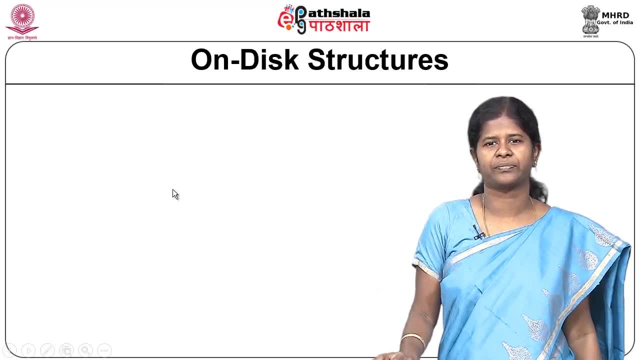 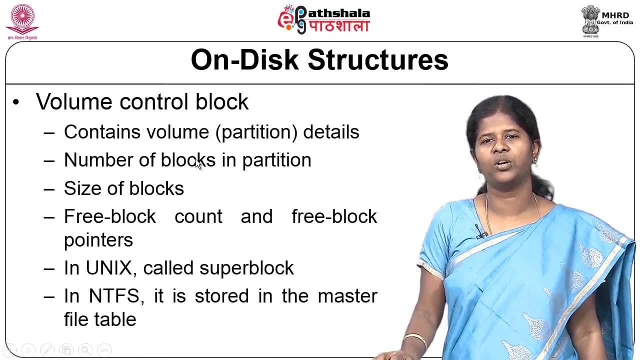 is called a partition boot sector. So this is one structure that is being maintained to help in booting an operating system. And then we have the next data structure, called a volume control block. This has information about a particular volume or a partition. What kind of information? 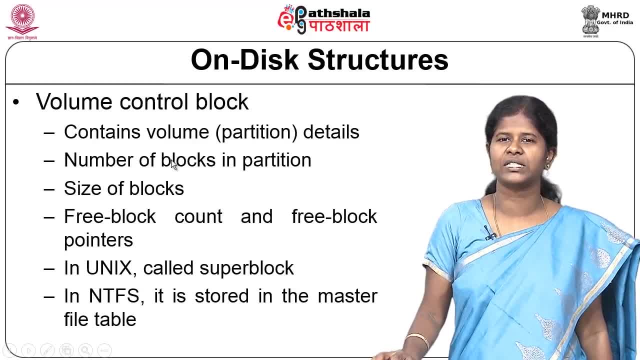 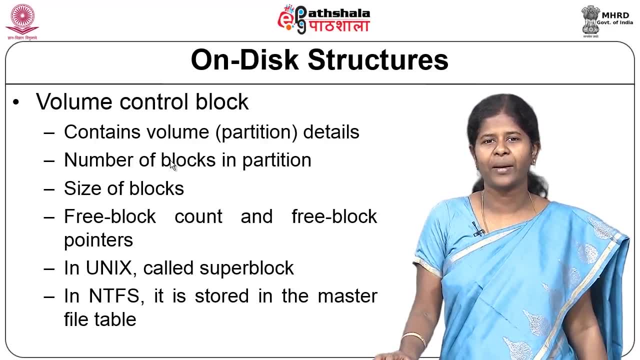 That partition will have many number of blocks, So the total number of blocks that are kept in that partition, Then what is the size of each of those blocks And, if there are free blocks, the number of free blocks that are maintained in that partition, and it will also. 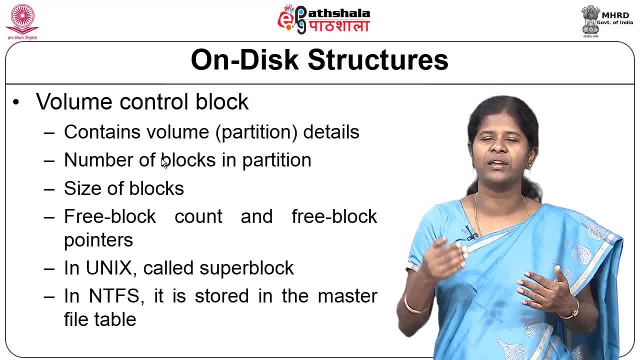 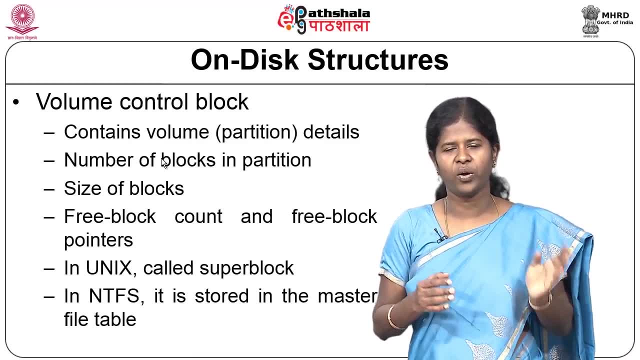 have pointers to the free blocks or it will have the addresses of the free disk blocks. All these will be maintained in something called a volume control block. In the case of UNIX, following that boot block, you will have a disk block which maintains this information call, which is called super. 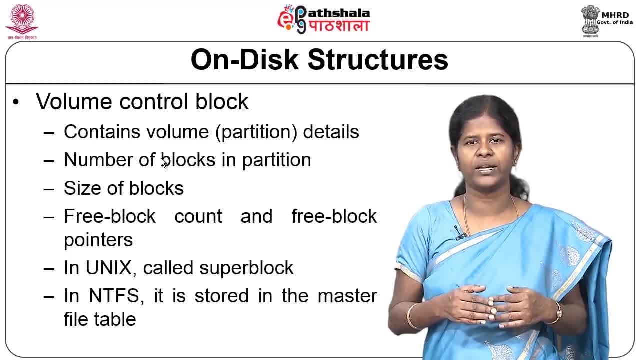 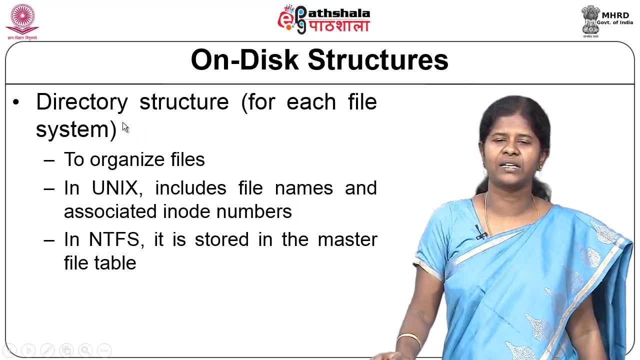 block. In the case of NTFS, this is stored in the master file table. Now the next structure is the directory structure. This directory structure is for each file system. So, as we all know, the directory structure is used to organize files. We will have directory. 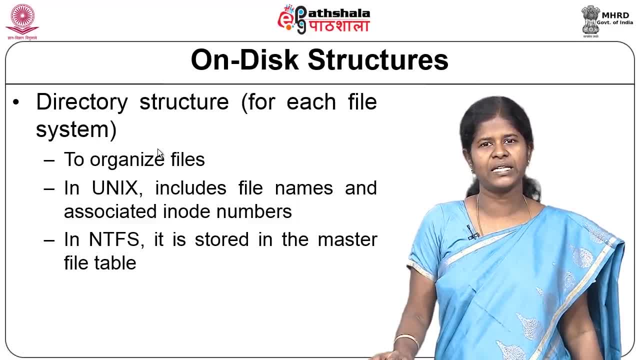 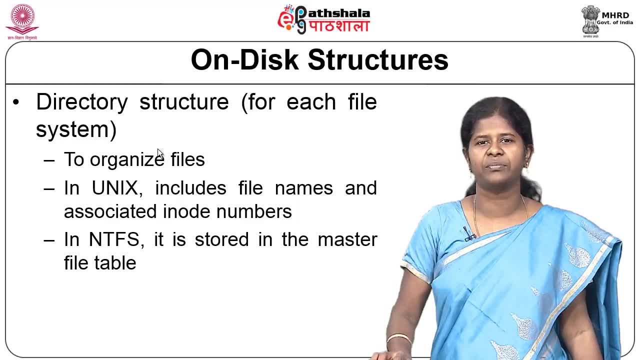 subdirectories beneath it, files beneath it and so on. And what happens In a case of on And what is maintained in each of the directories? The name of the file is maintained and also the associated information will be kept In the case of UNIX, if you see that, 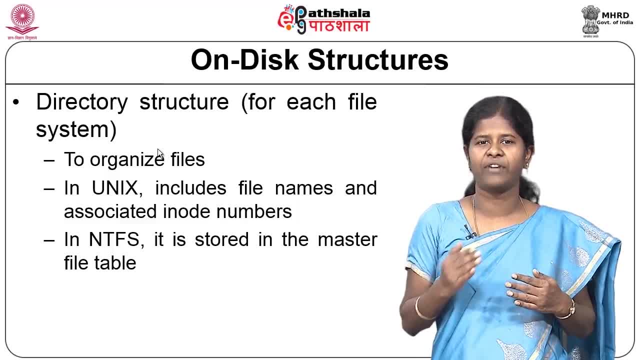 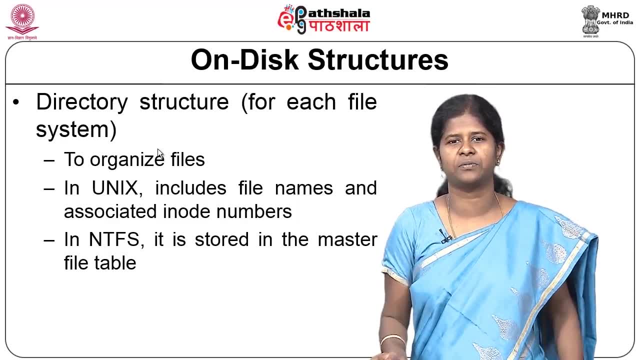 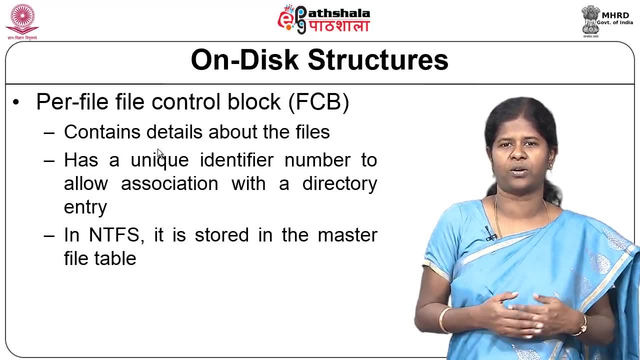 the names of the files and the inode numbers of those files will be kept in each directory entry. In NTFS this is stored in a master file table. And then one more structure we have got, which is called the per file file control block. 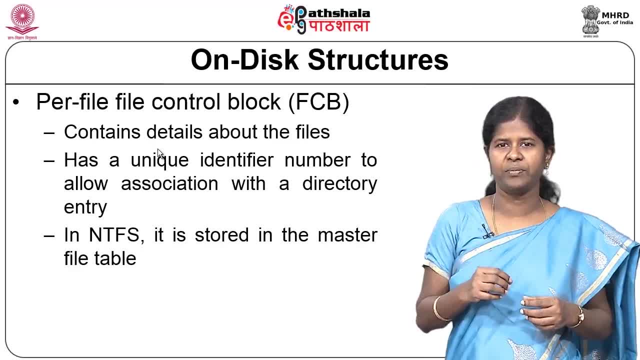 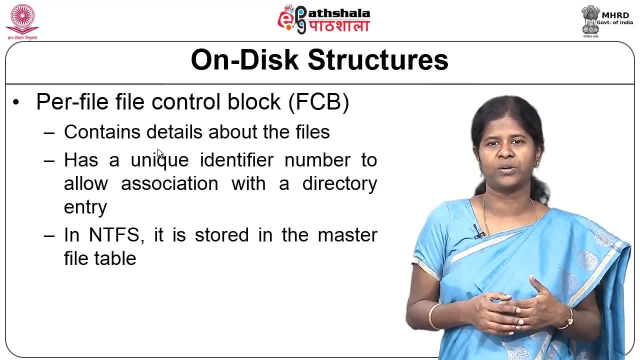 So for each and every file, metadata about that file should be maintained in some place or just maintained in a file control block. As I told you, in the case of UNIX it is maintained in an inode. So what metadata will be kept in these files It will have all details about. 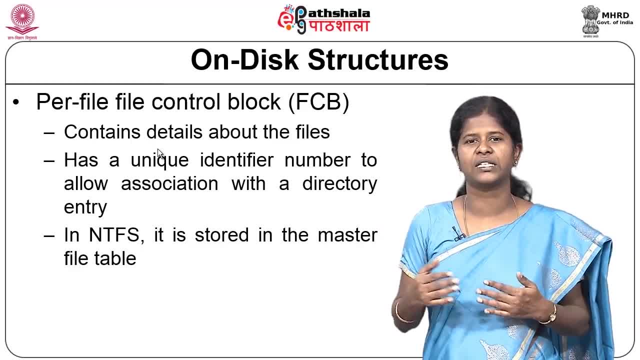 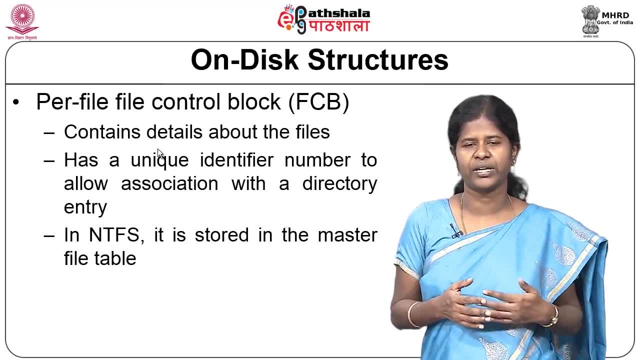 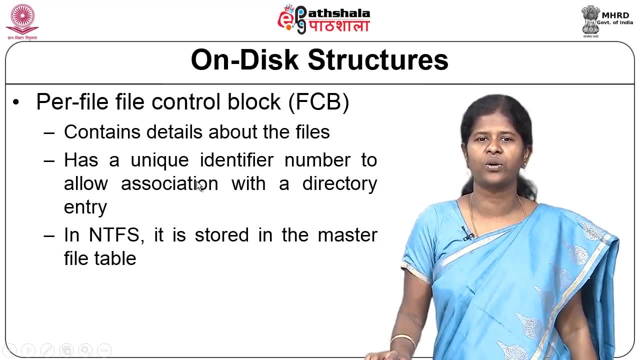 the files, like the owner of the file, the size of the file, etcetera and so on. And then it has a unique identifier number to allow the association with a directory entry For inode. there is an inode number In NTFS. this per file file control block is stored. 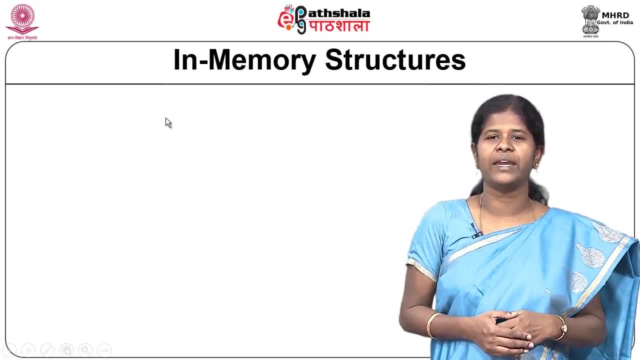 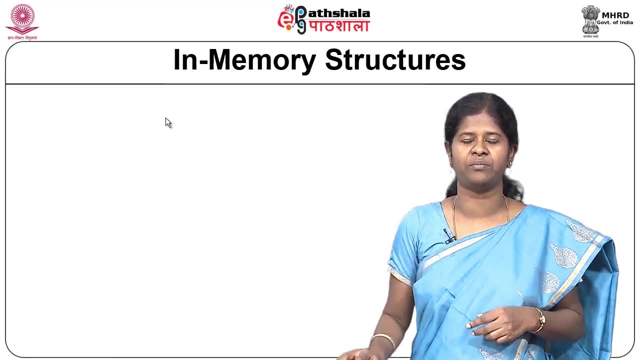 in the master file table. Now we will see different in-memory structures that are maintained for the implementation of the file system. There is structures that are maintained within the main memory for the implementation. One is a mount table. We have learnt about this. 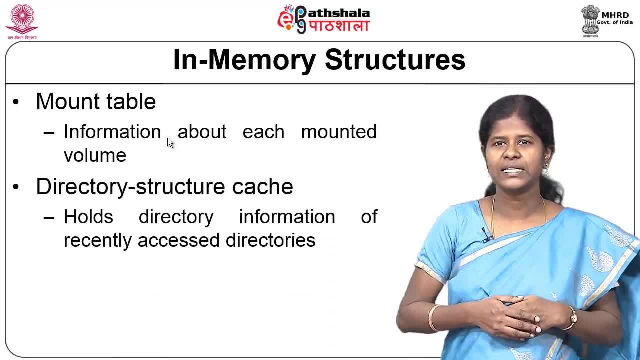 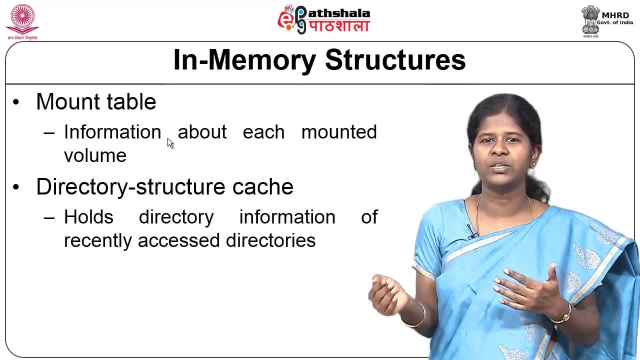 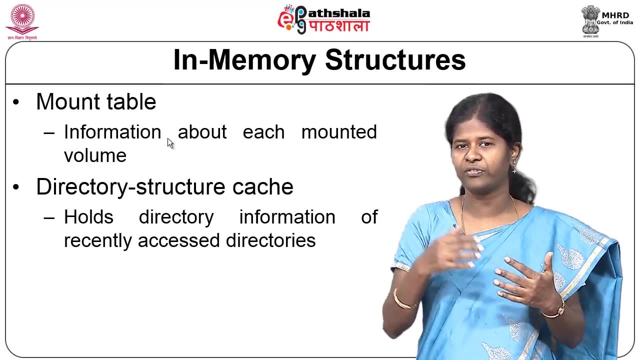 mount table in an earlier module. That is, when you want to logically attach one file system to another- file system 10- Then information about this mounted volume is maintained in this mount table. The mount table have information about the directory onto which the new file system is logically. 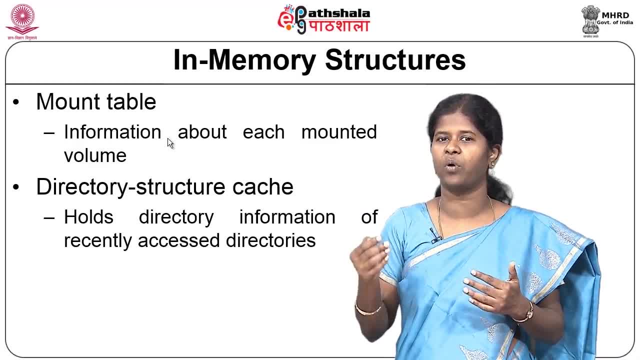 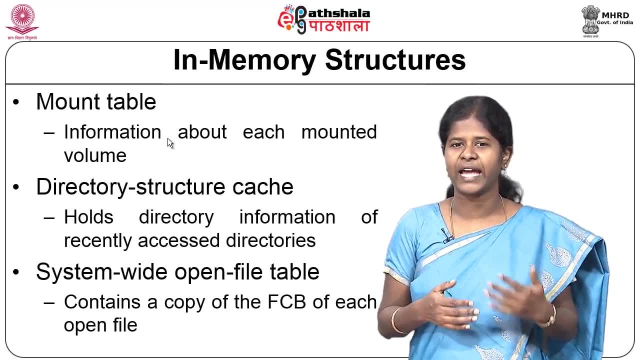 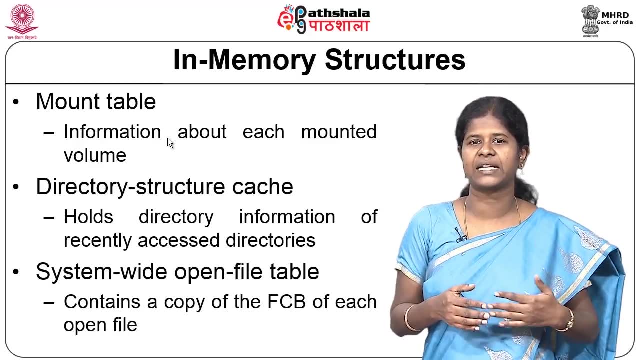 attached to and the device file name of the mounted file system. All these will be maintained in a mount table. The second structure is a directory structure cache. This directory structure cache: it holds the directory information of recently accessed directories. So if you want to access the same directory contents again, then you do not have to read. 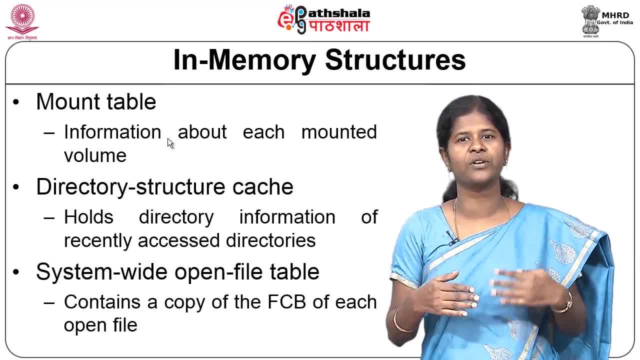 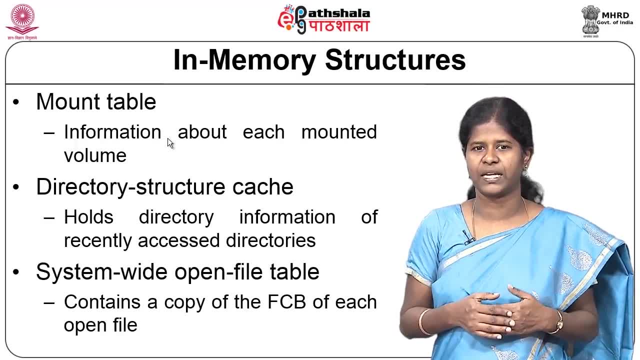 from the disk and then access the contents. You can just make use of this cache, look into the cache and get the information about the directory- may be the contents of the directory- from the cache itself. 11. Then we have something called the system wide open file table. This is a common file table. 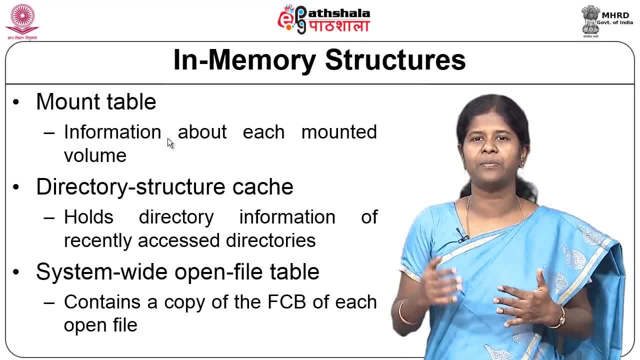 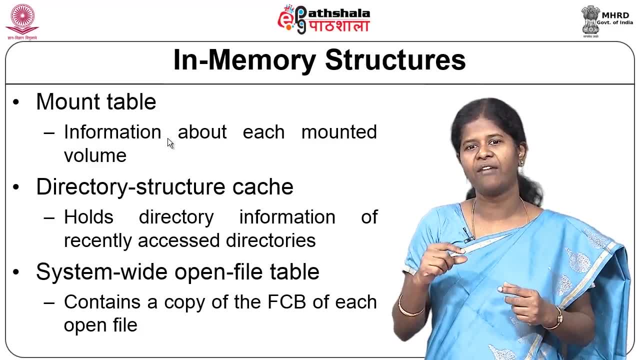 that is being maintained for all the processes that are present in the system And these. the entry of this open file table will have information about the FCB of each file. Where does the FCB? it is the file control block. Any case of UNIX is the I know or it will. 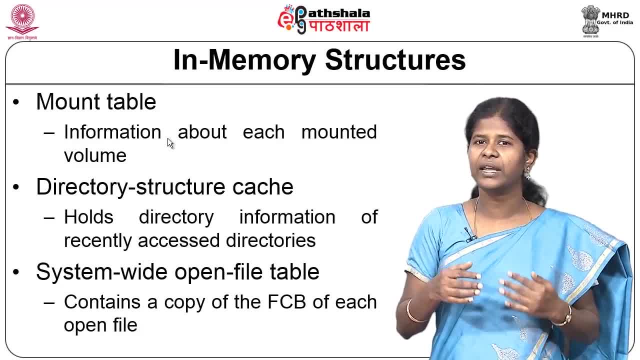 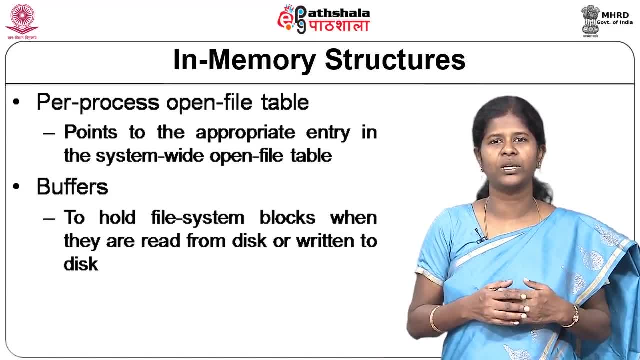 have the metadata of the file, So that is kept in this system wide open file table. and then we have something called a per process open file table 12. The system wide open file table has got entries for all the processes that are present in. 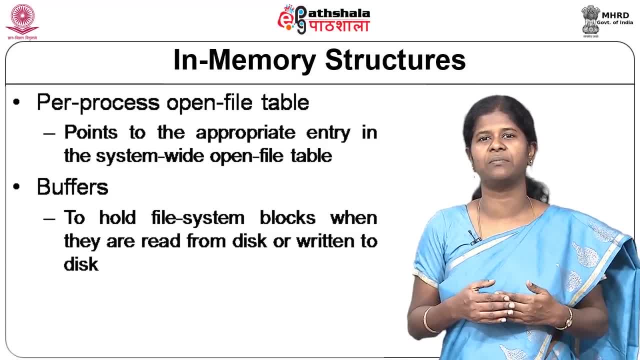 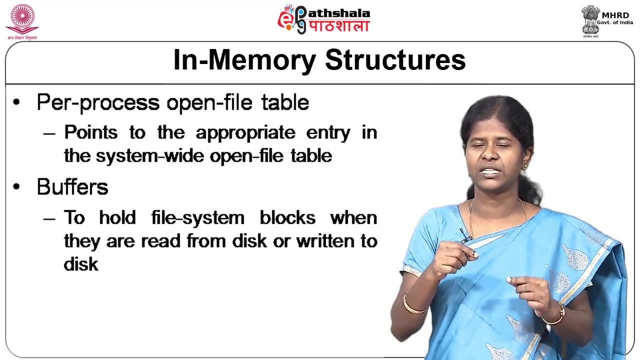 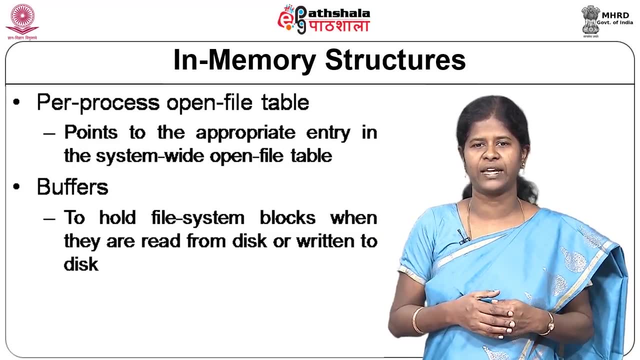 the system 10 per process. open file table. you have a file table- open file table for each and every process, So this will have information about the files that are opened by that particular process And the entry here will point to the appropriate entry in the system wide open file table. 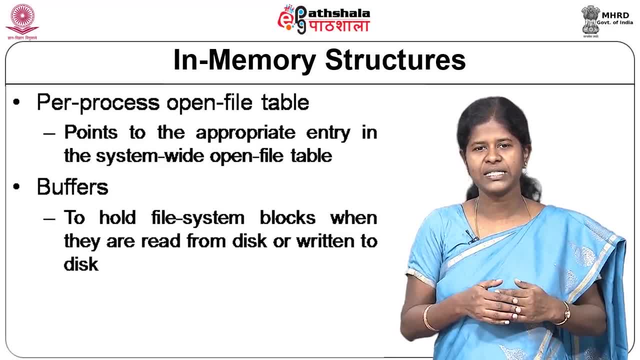 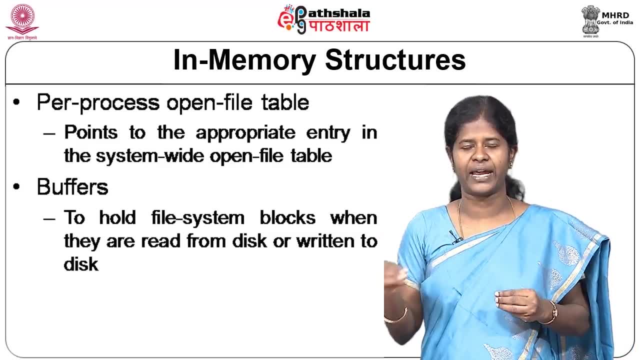 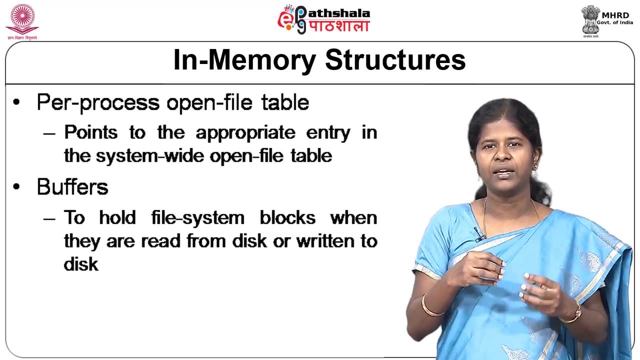 And then we have buffers. So these are buffers that are kept in the memory to hold the contents of disk blocks. So disk blocks have the contents of files and when you are reading a file from the disk you store the contents of the file in this buffer that are kept in the main memory. 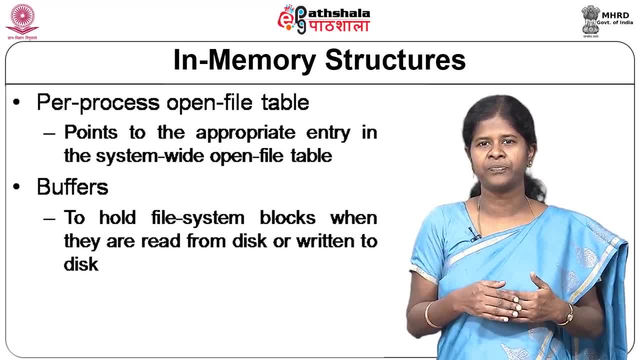 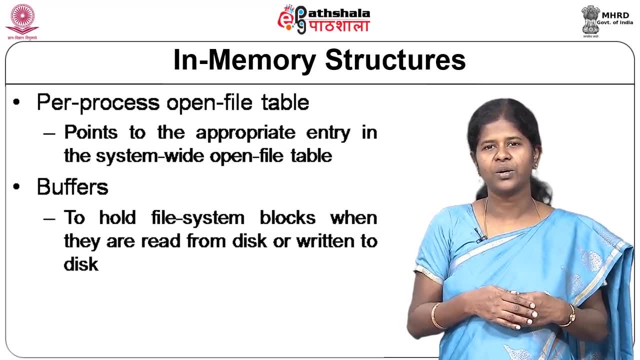 So the next time, if you want to access the same files contents, you can read it from these buffer rather than reading it from the disk the second time. So even if you are writing to a particular disk which is a part of a file, you can write. 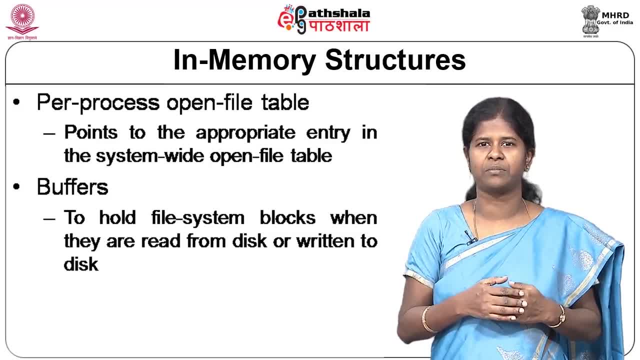 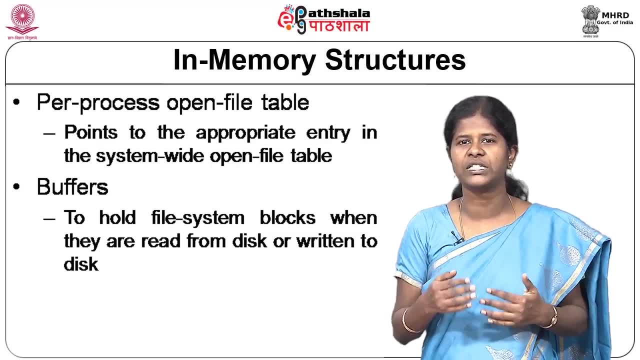 to these buffers And the writing can be delayed for some amount of time. So you may be can read from a particular block, you can write into the block again, read, write, etcetera, and so on. So changes, a number of changes can be done to a particular block of a particular file. 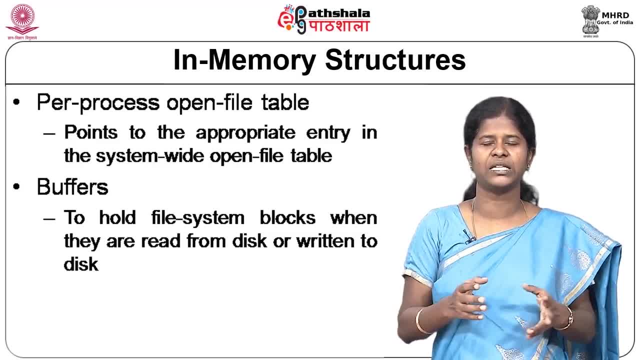 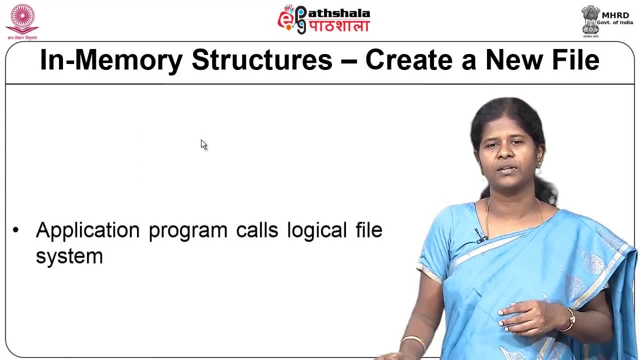 But you do not have to write it each and every time to the disk. you can maintain it in the main memory in this buffer And after all updation have been done, then you can write it back to the disk. So now we will see how these structures have been used when a new file is created. 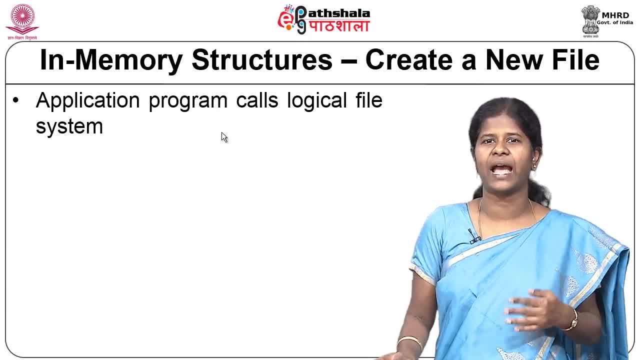 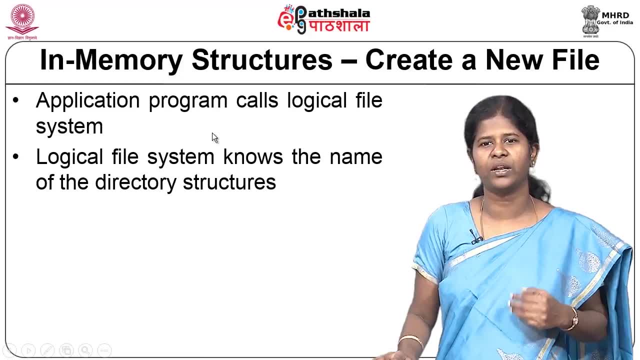 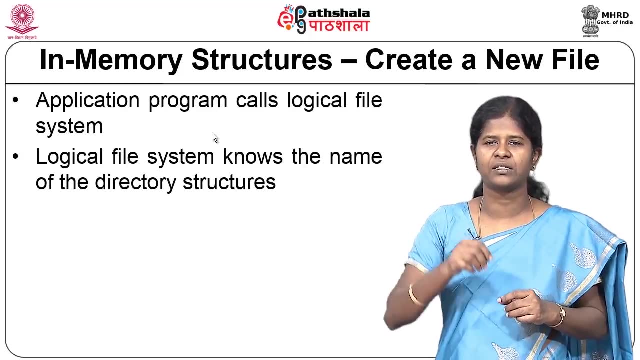 So we saw that the top most layer in the layered file system is the application program. The application program will call a logical file system. The logical file system will know that name of the directory structures. here we need to create a new file. so the application will say that a file with name say, say abc, has 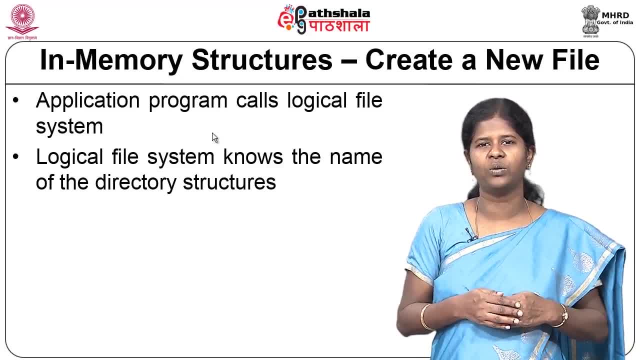 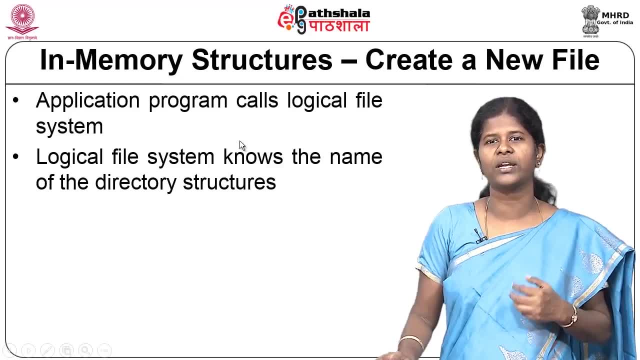 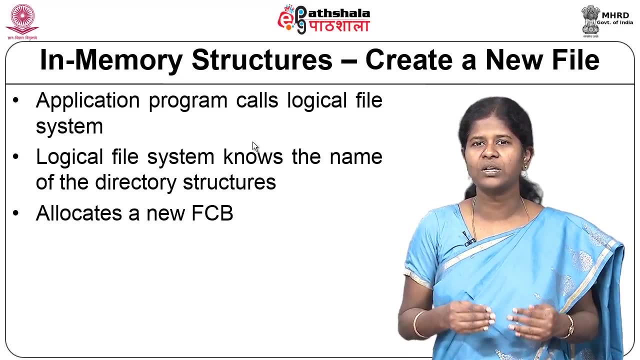 to be created. So now the logical file system will know the directory structures, so it should know the parent directory where this particular file has been created. ok, has to be created or it will be created in the current directory and a logical file system will allocate a new file control block because a new file has to be created, a new FCB will. 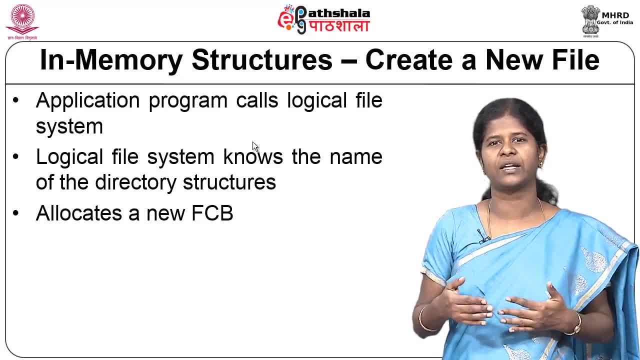 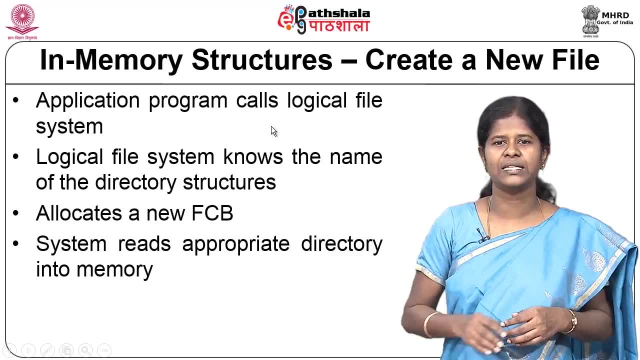 be assigned for this file. In the case of UNIX, the FCB is nothing but an inode, So an inode will be assigned or will be allocated for this new file that is been created, and then the system will read the appropriate directory into the memory. 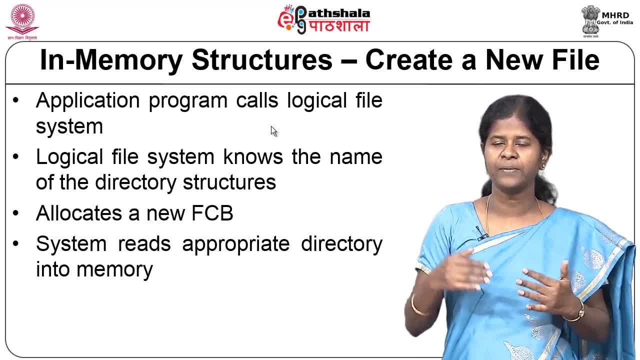 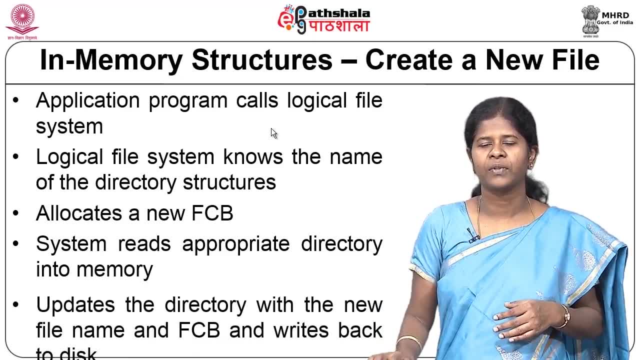 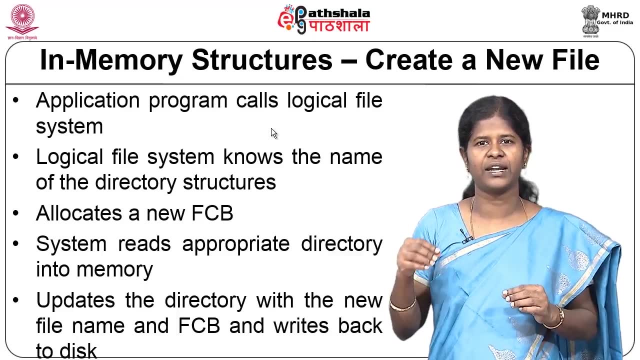 And if you are trying to create this file in the current directory, then the current directories contents will be read into the main memory. Now what we need to do: In the directory, you need to create an entry for this new file and the data related to that. 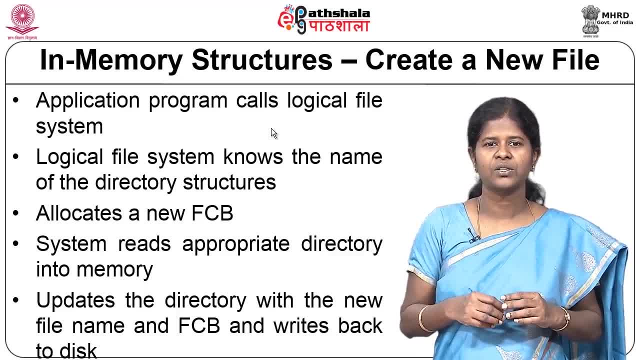 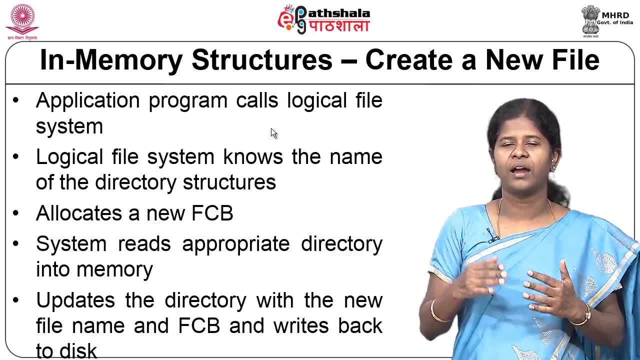 FCB has to be written in that particular directories entry. So you know the directory, So you have read the directory from the disk into the main memory. Now, in this directories contents, you need to create a new file. So you need to write the name of the file and the FCB. and once this entry is been made, 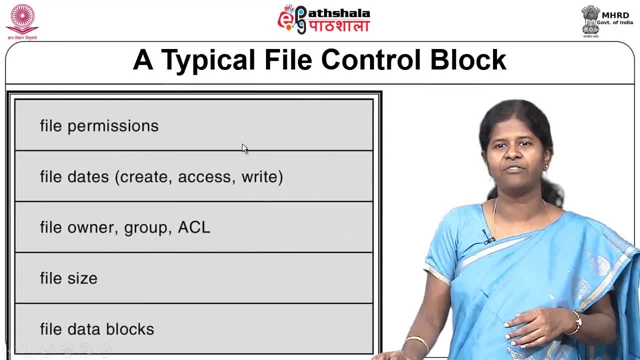 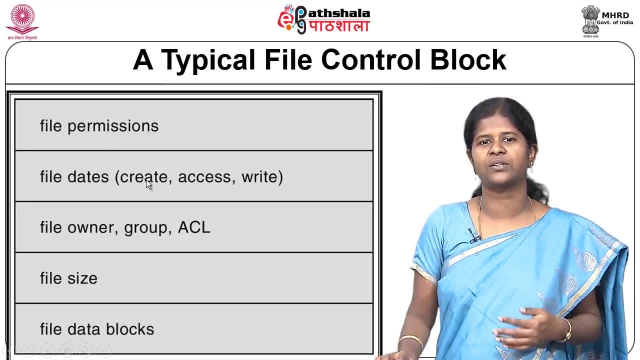 this directory can be written back to the disk, So a typical file control block will look something like this. You will have file permissions, file dates, when it was created, when it was accessed, when it was written, etcetera and so on. The owner of the file. 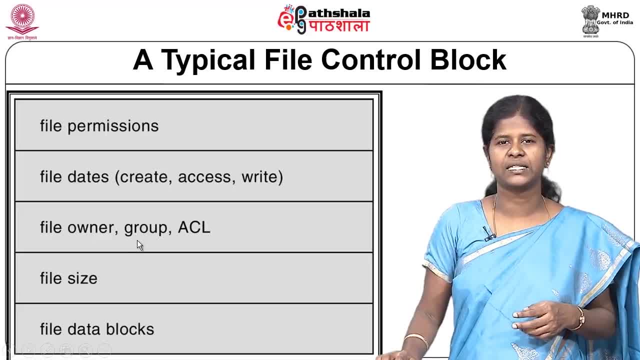 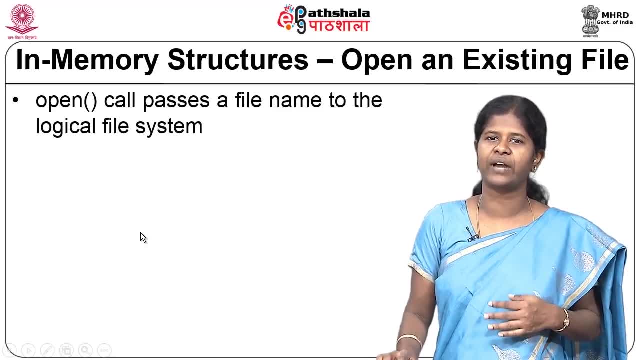 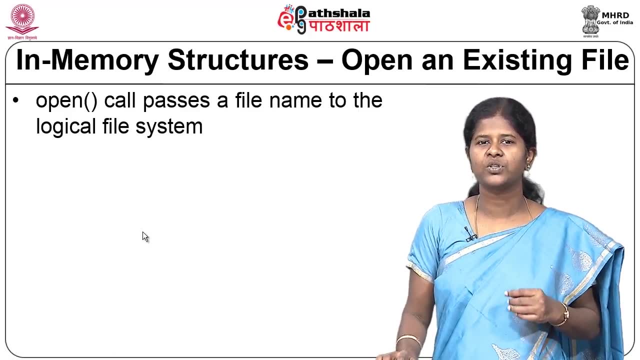 the group, the access control list, the file size, the data blocks and so on. All these will be kept in this FCB. So now we will see what happens when an existing file is to be opened. So the open call given by the application will pass a file name to the logical file. 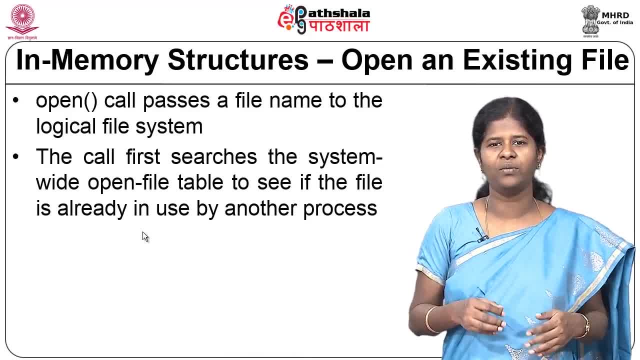 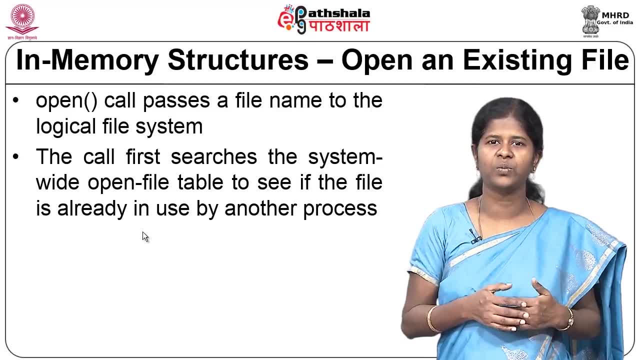 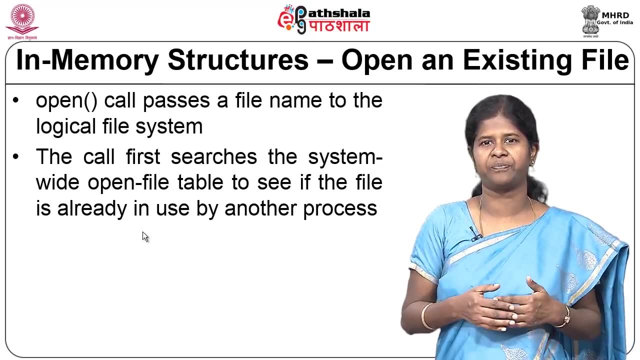 system the name of the file which has to be opened. This call will first search the system wide open file table to see if that file is already in use by another process. It may be possible that the file is opened by another process at the same time. So, looking into the system wide open file table, it will 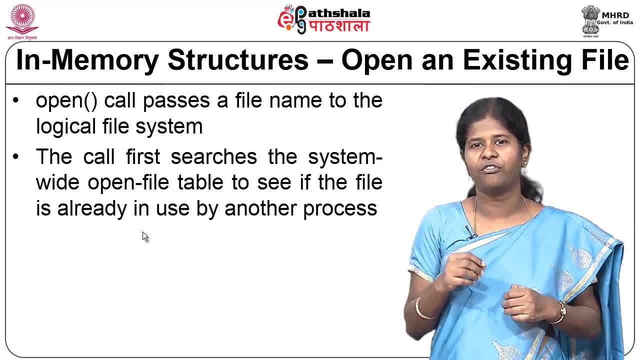 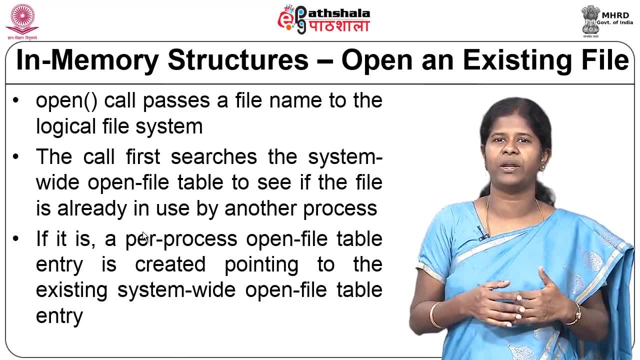 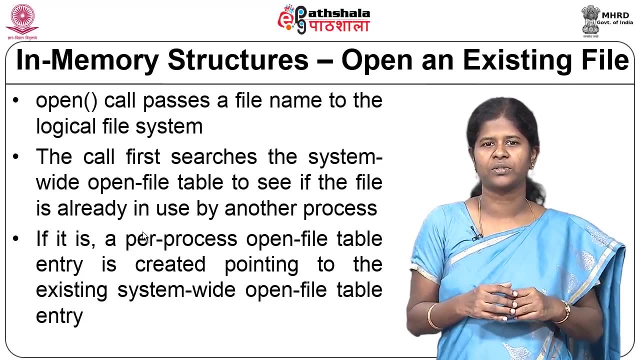 find out if there is an entry for that process, for that file, by some other process. So if there is an entry, then it means that the file has been opened by another process. So the same entry in the system wide open file table will be used by this process also. 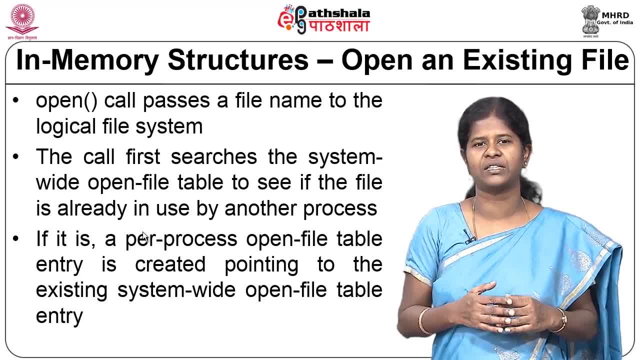 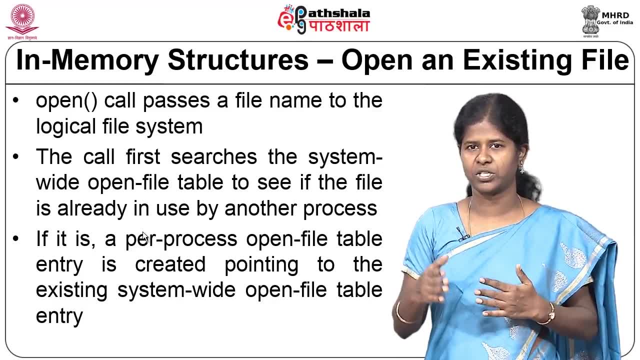 So it will create a per process open file table entry for this file, because this is a different process that is opening that file. So for this process there will be a per process open file table in that an entry will be created and from that entry a pointer will. 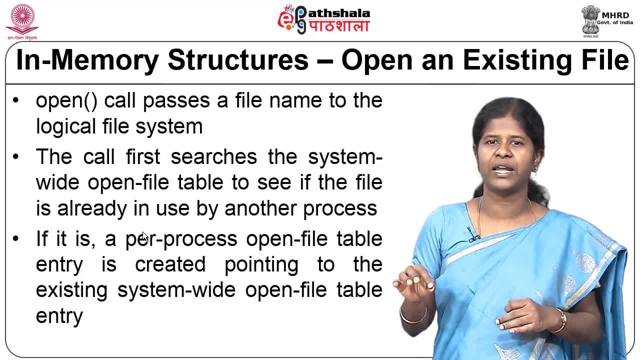 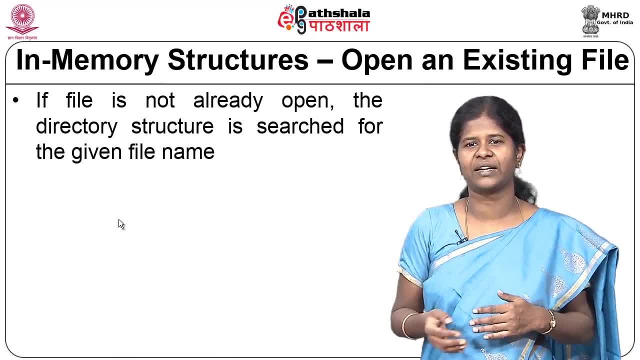 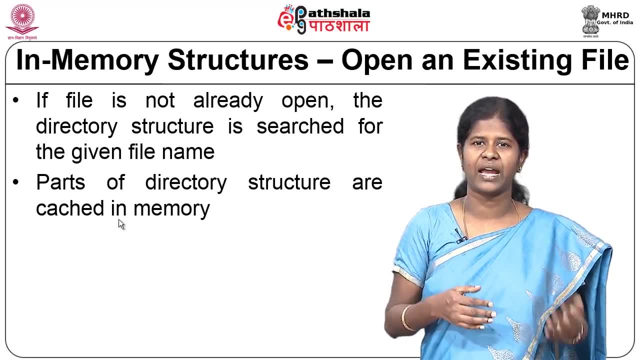 be made to point to that system: wide open file table entry which is already existing. If the file is not already open, then you need to search in the directory for the given files name and it is possible that part of the directory structure can be cached and kept in memory. 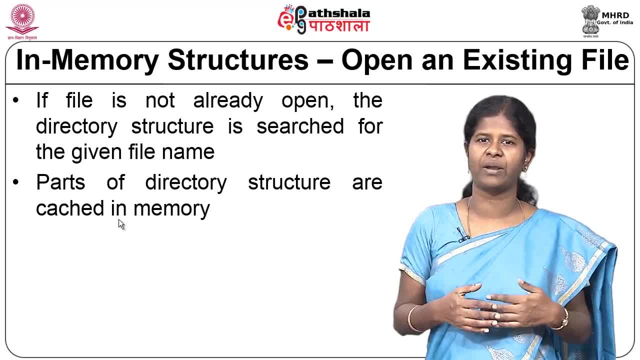 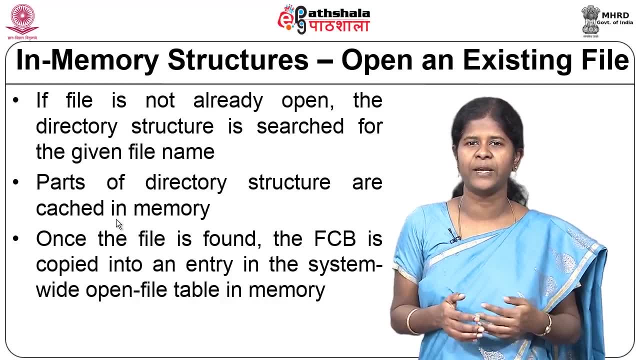 as I told you earlier. So if it is present in the cache then you can read from there, or you need to read from the disk. So once the file is found in the directory's contents, so you read the directory and search into the directory to find the contents of that file- there will be an entry in the directory. 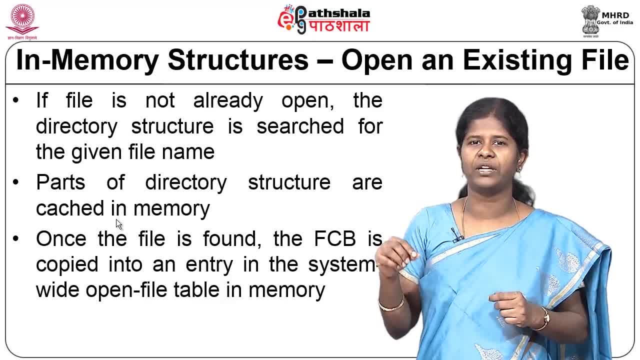 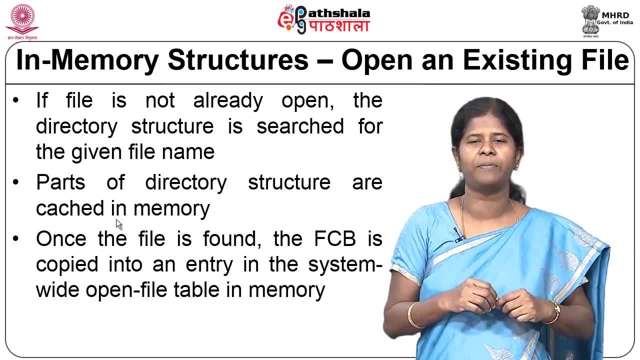 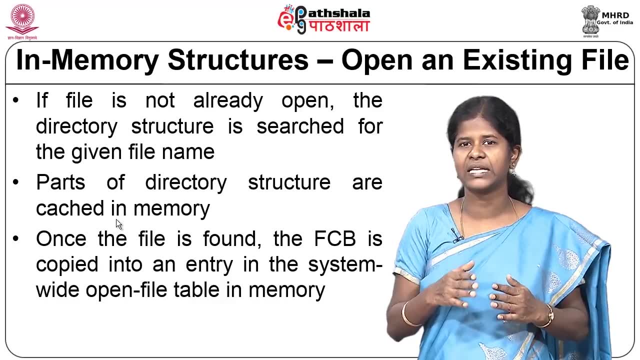 for this particular file and the FCB is also kept. the information about the FCB is also kept in the directory's entry. So now you get information about the FCB and the FCB is now copied into a new entry in the system wide open file table, because the system wide open file table in this case does. 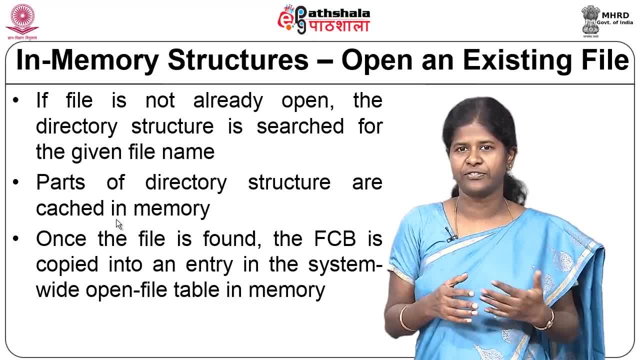 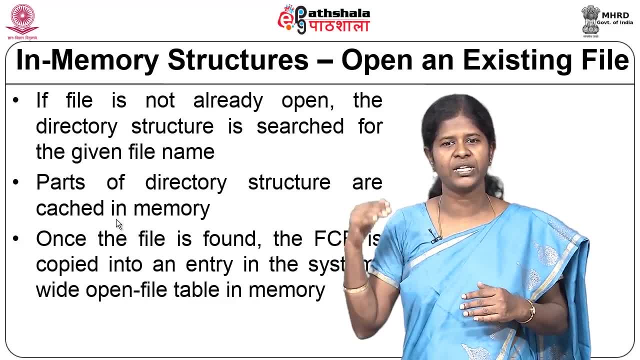 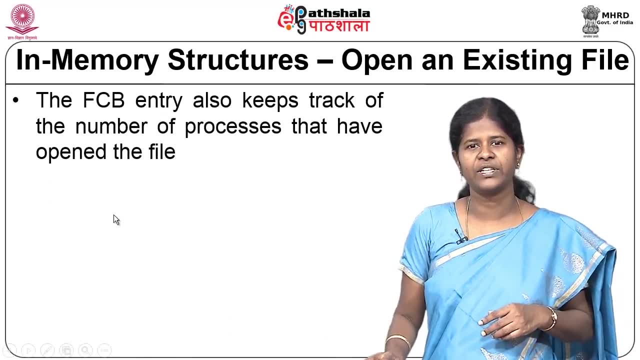 not have an already existing entry. You are creating an entry for the first time, So you need to get hold of the FCB of the file from the directory and make an entry in this system wide open file table and copy the FCB into the system wide open file table So the FTB entry will also have information. 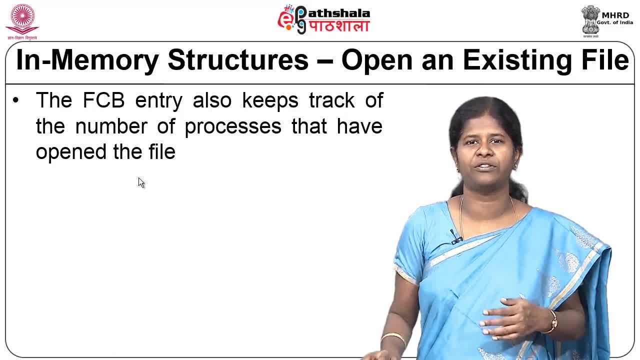 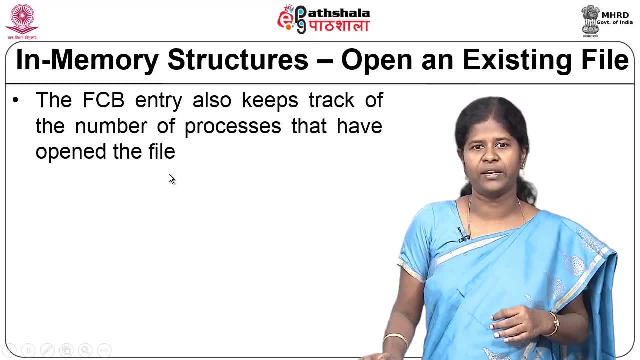 about the number of processes that have opened the file. that is, in the file table entry. You will have the count of the number of processes that have opened the file And now an entry is made in the per process open file table. this entry is made to point. 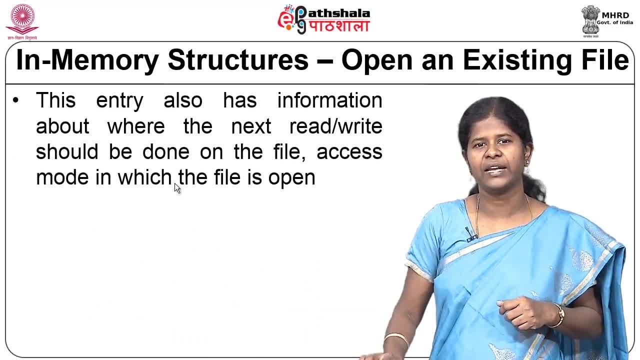 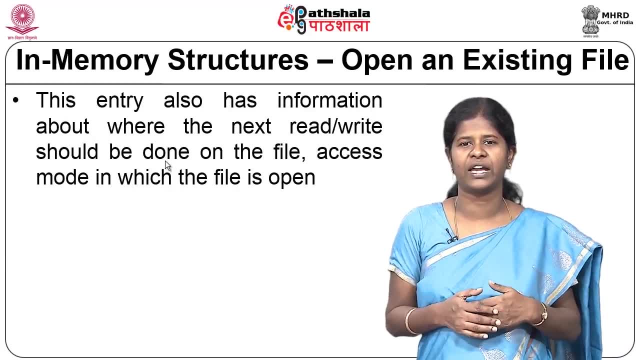 to the system wide open file table. So the entry will also have information about where the next read write should be done on the file, the access mode in which the file is open and so on. So the system wide open file table entry has information about the number. 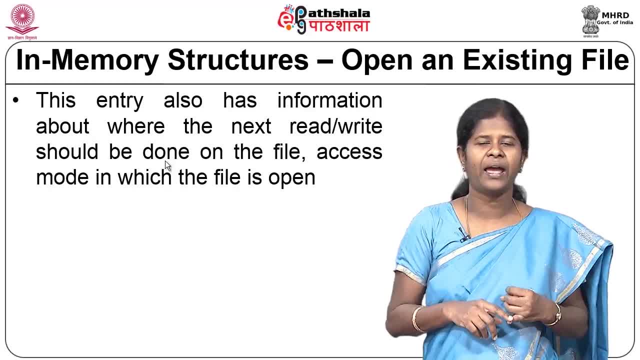 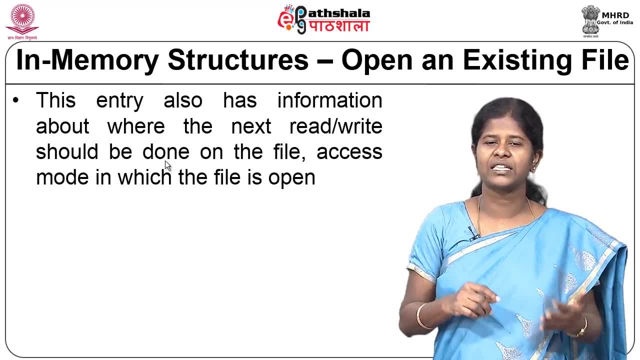 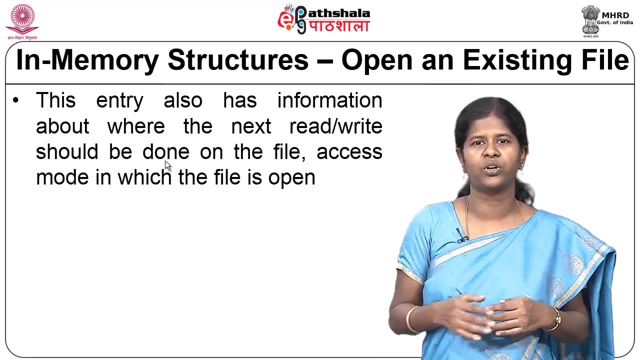 of processes that are using that particular entry and the offset within the file where the next read or write should happen file and the access mode in which the file is open, say whether the file is open for read only mode or write only mode, or read write mode and so on. All those information will 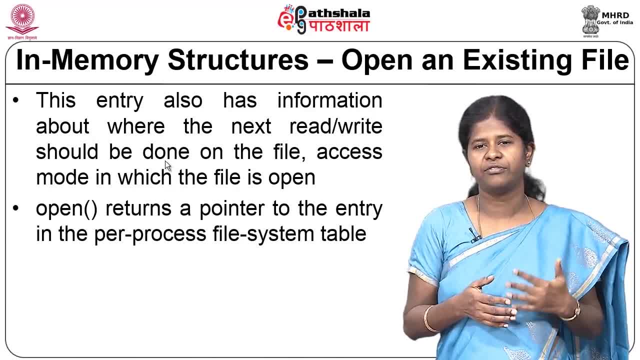 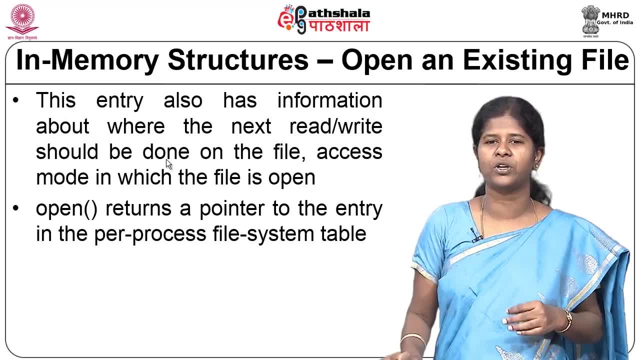 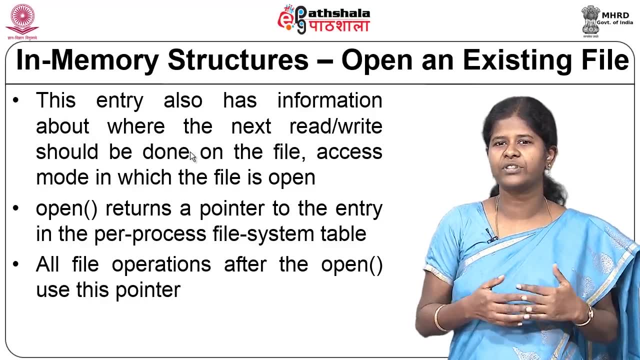 be kept in this, in this file table entry And finally, what is returned is the open will return a pointer to the entry in the per process file system table. So after this, all file operations that are be done after the open, you will have to read: 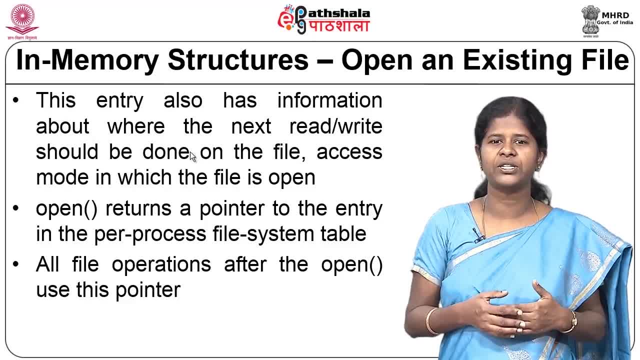 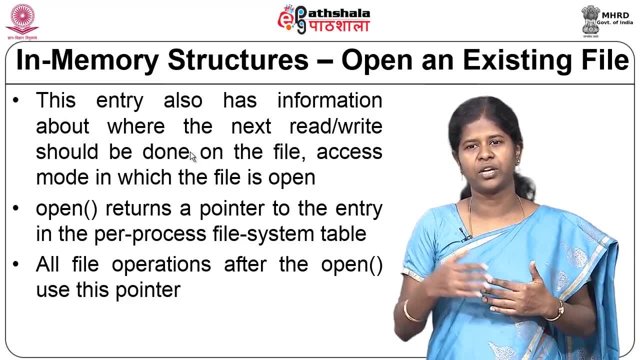 from the file you may have to write into the file and so on. So all file operation operations that have been done will use this pointer to access the per process file system table and thereby it can make use of the system wide file table entry, which will have the 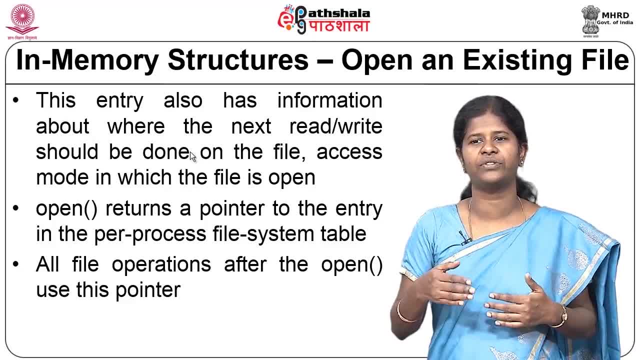 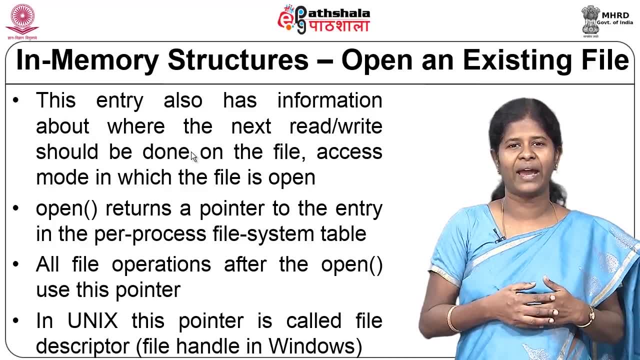 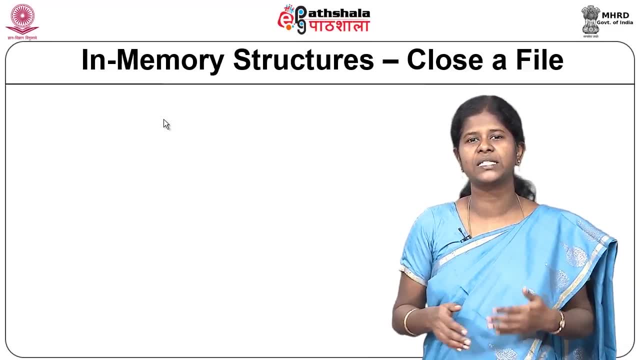 FCB. FCB will have information about the location of the contents of the file in the disk. In UNIX this pointer that is been returned is called a file descriptor and the case of windows, this is called a file handle. This means when a file is closed, how the structures are being used When a process is closing. 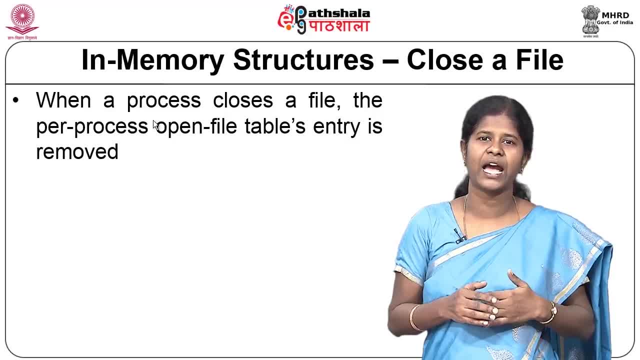 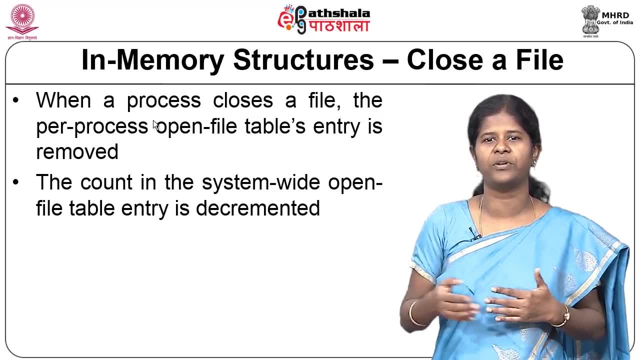 a file, the per process open file tables entry has to be removed because the file is no more going to be used by the process. But there is a pointer from here to the system wide open file table. So you use that pointer to the system wide open file table and access. 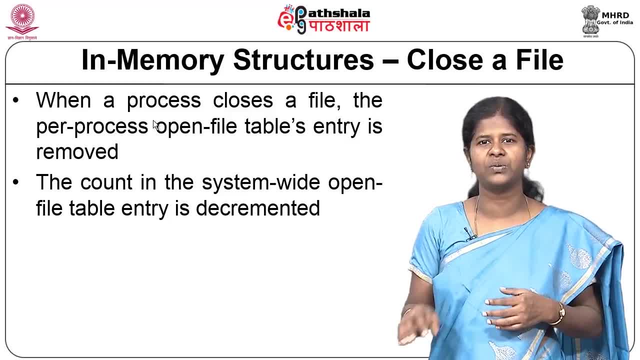 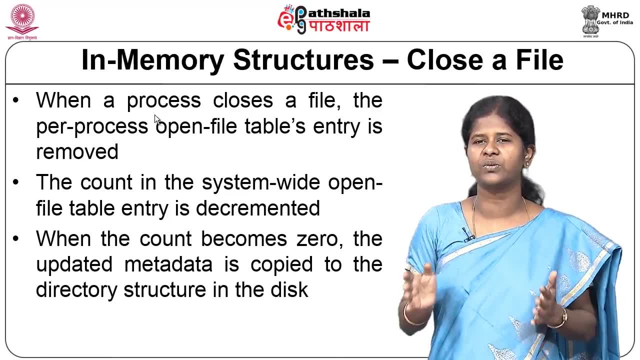 that entry and try to find out the number of processes that are using that particular file, So that count is decremented If the count becomes 0. So that means that no process is using that file as of now. only this was the one process. 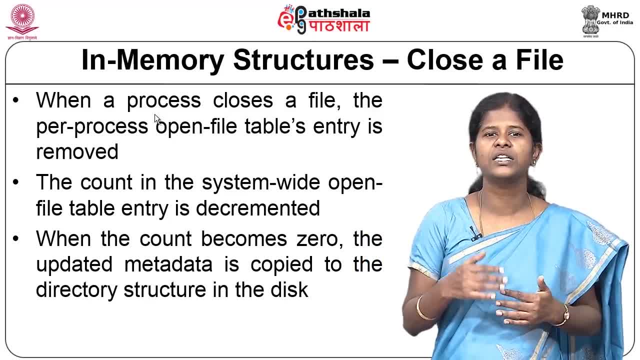 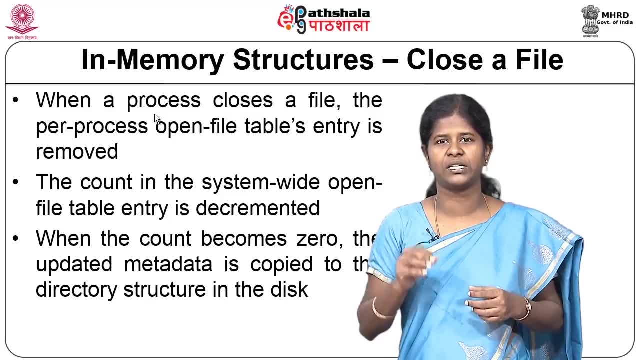 that was using And hence the updated meta data is copied to the director structure in the disk. So you had something called an FCB that was maintained in the entry, which has got information or meta data about that file. All these information are copied on. 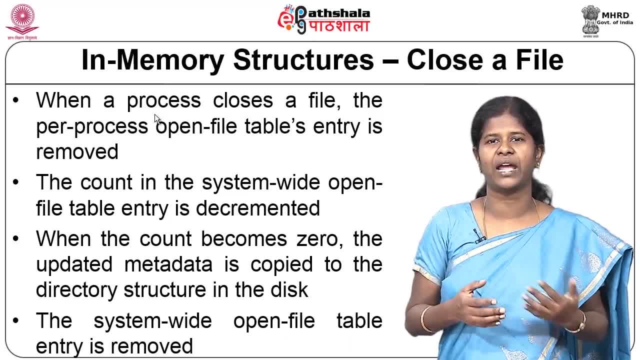 to the disk. The system wide open file table entry can be removed now because the count here is 0. No other process is using this file as of now. So here you can look at this diagram here. So that is the file that is being used to. 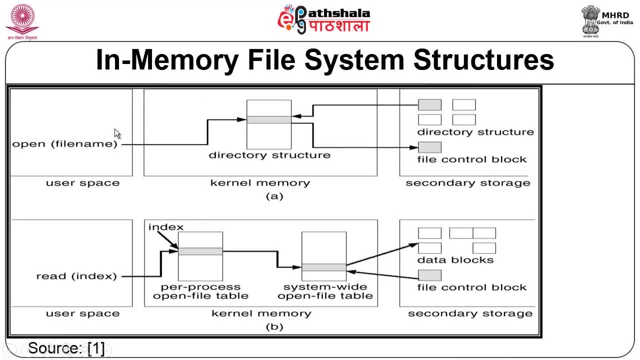 build the system wide open file table entry. So this is the file which is called the fcb diagram. you can see that the user is providing open of a file name, which means that it needs to access the structure of a directory And the structure of the directory can be kept. 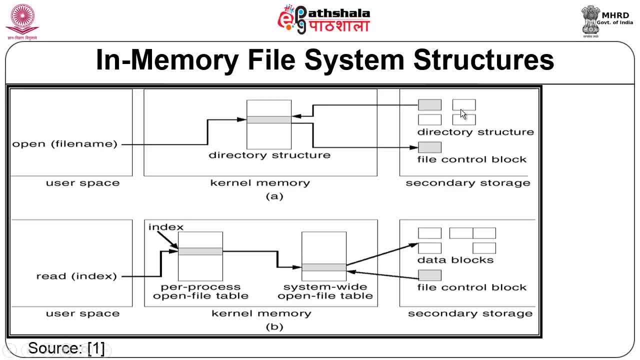 in the disk is actually kept in the disk, So from there it can copy it into the kernels memory and from there you can access the file control block And then say: if you want to read from a file, so you need to read, provide the index This. 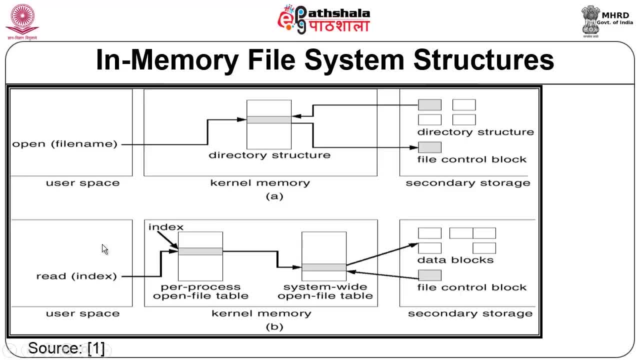 index is actually a return of this open call, So that index is used to access the per process open file table entry. From there you follow the pointer to the system wide open file table entry and then from there you can access the FCB And the FCB will have details about the. 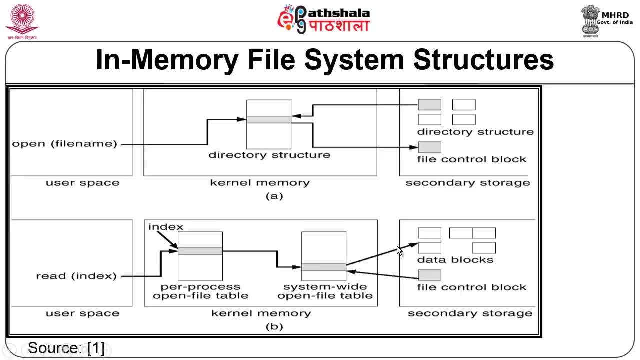 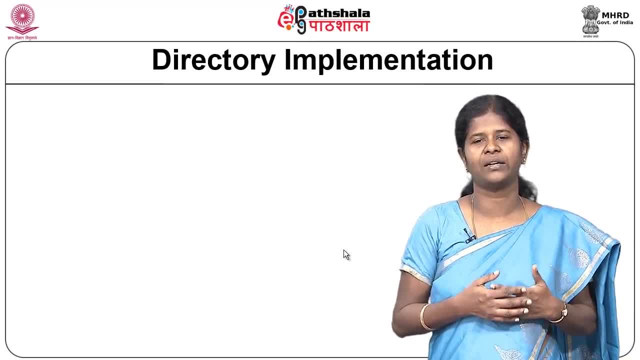 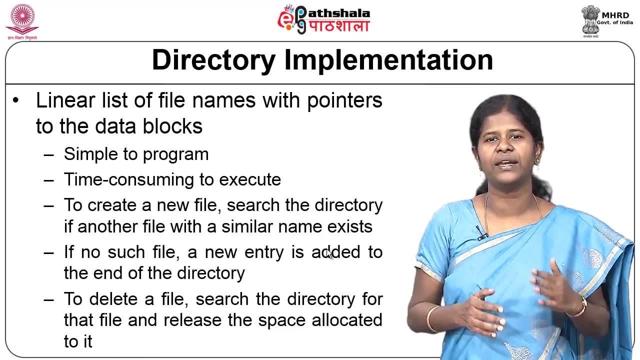 address of the disk, And this blocks which contain the data in the disk. So now, having seen this in memory structures, we will look at how directories can be implemented. So the simplest way to implement a directory is to have a linear list of file names and 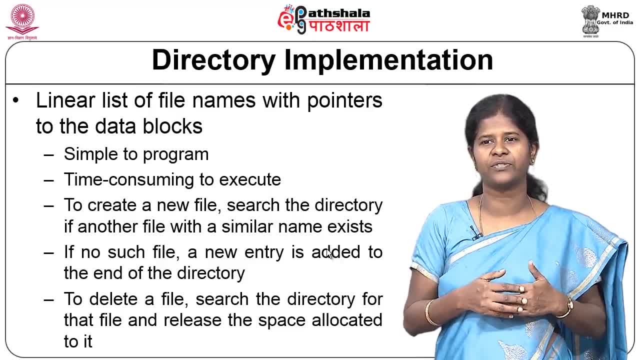 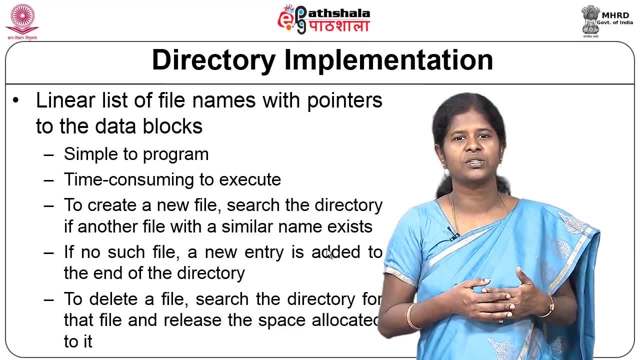 that can have pointers to the data blocks where the contents of the file are kept in the disk. But this is very simple to program but the problem is it is very time consuming To execute, that is, to create a new file. you need to search the directory if another file 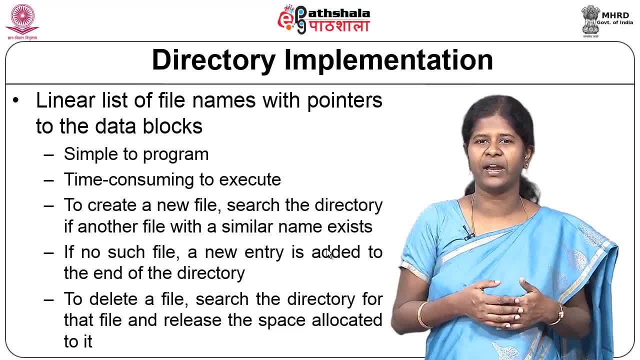 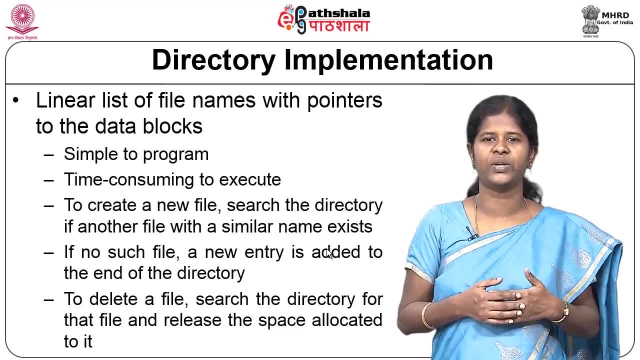 is present with the same name. If there is no such file of the same name, then a new entry has to be added to the end of the directory, And to delete a file you need to search the directory for that file and release the space that is allocated to that file. 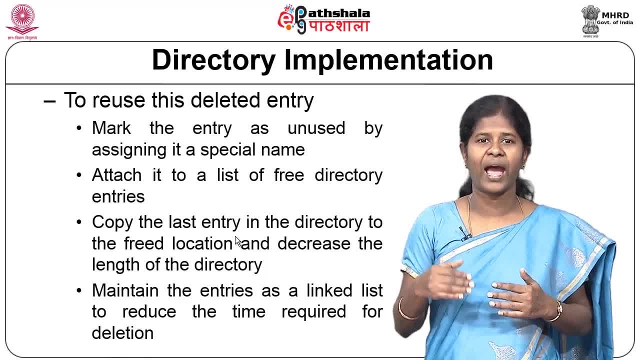 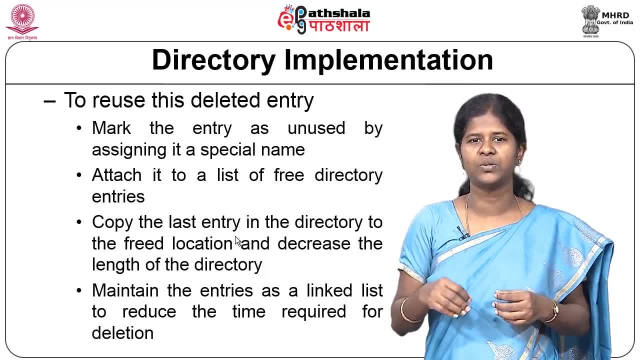 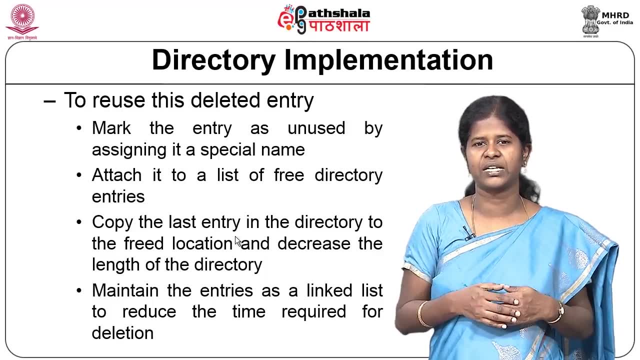 But now, when you delete this entry, you have to, you have to you reuse this deleted entry. How do you reuse the deleted entry? You can mark that the entry is unused by assigning it a special name, or you can attach it to a list of free directory entries or what you. 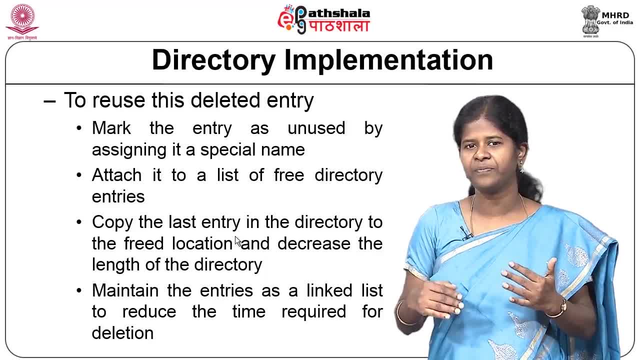 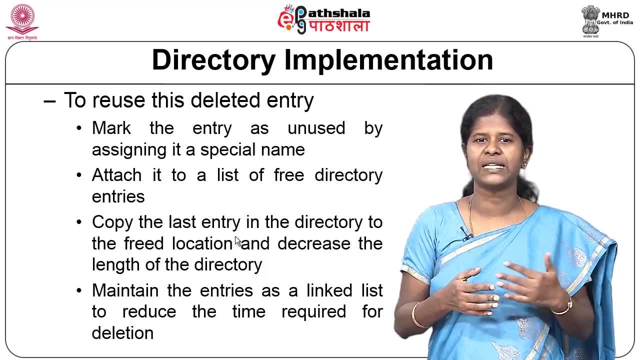 can do is that you can copy the last entry that is kept in the directory to this freed location and decrease the length of the directory. Or another way is to maintain the entries as a linked list so that deletion will become easier and it will reduce the time required. 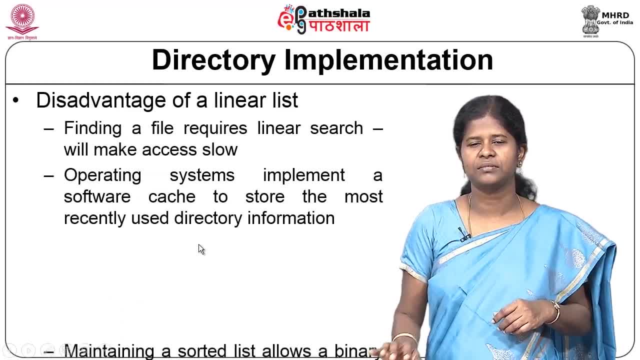 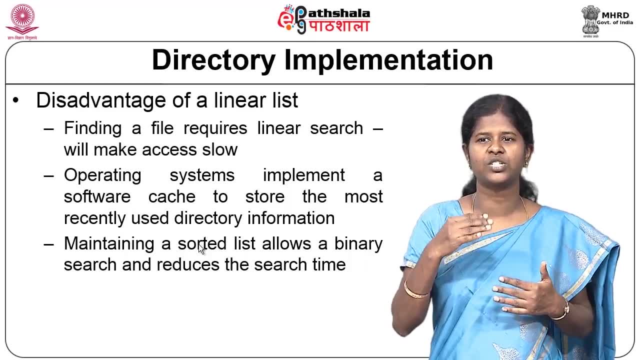 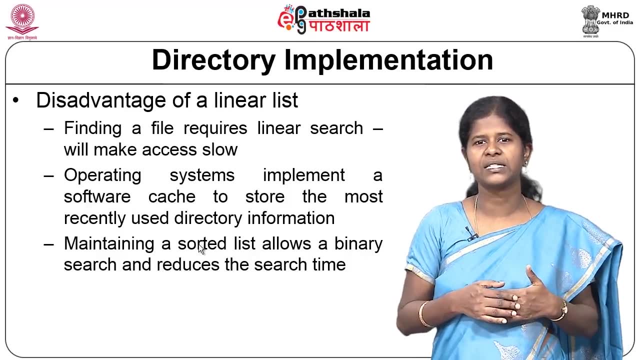 for deletion as well. But the disadvantage of having a linear list is that finding a file requires linear search, That is, you need to search one after the other to search for a particular file, which will make the access very slow, And operating systems implement software cache to store the most. 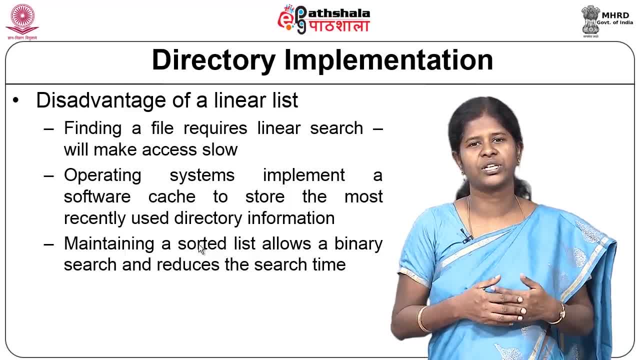 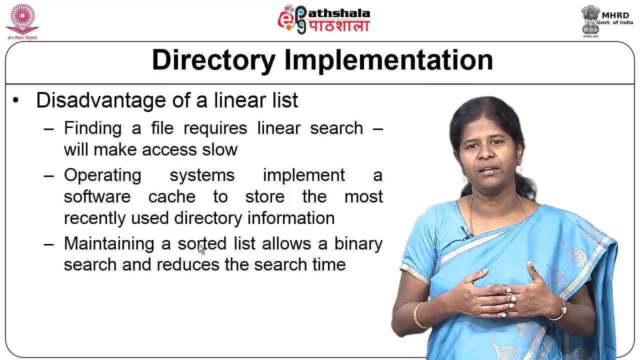 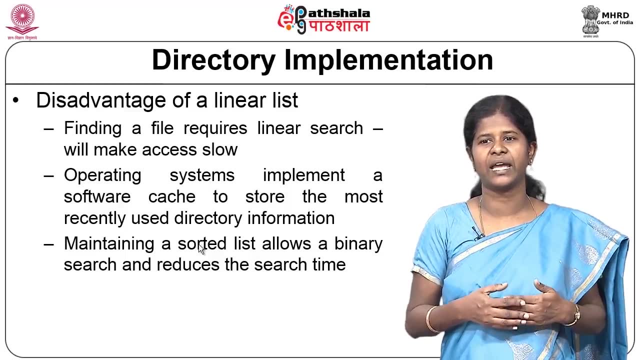 recently used directory information, which can make the search easier, And you can also maintain a sorted list And then allow a binary search within that list, which can reduce the time. But maintaining the sorted list again becomes difficult Whenever you are adding a new entry, then 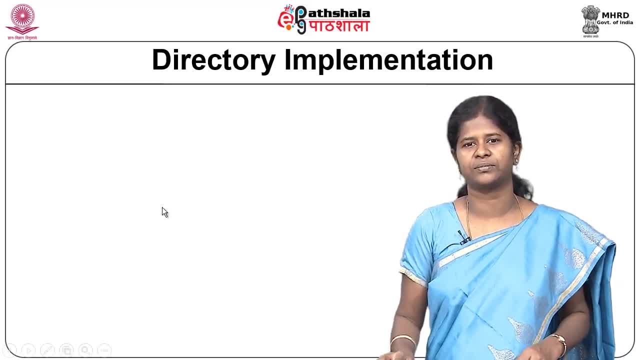 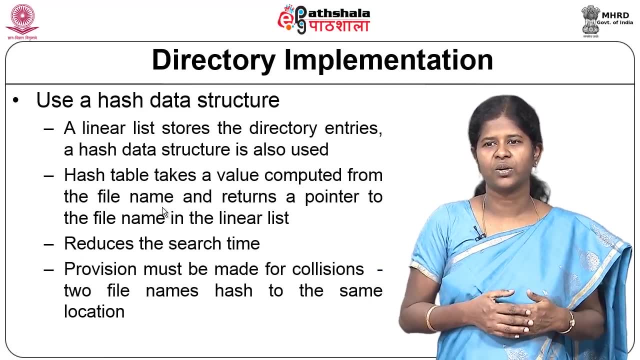 you need to ensure that the list is maintained as a sorted list. So, rather than having a linear list, you can go for a hash data structure. So you can have a linear list to store the directory entries, but you can have a hash data structure. 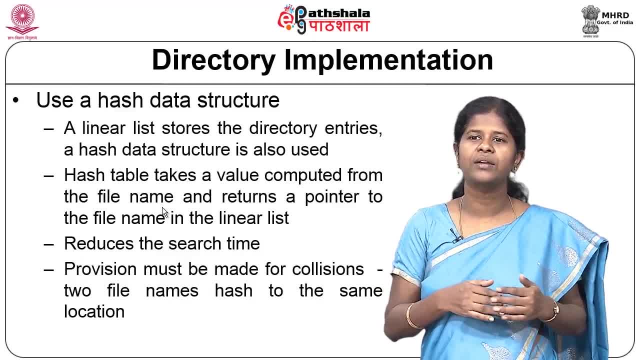 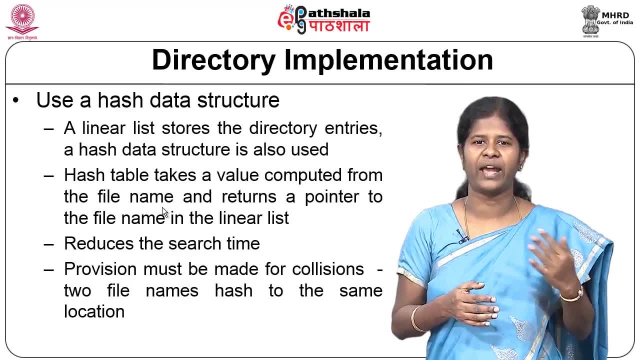 also, this hash data structure will help in pointing to the entries or getting the entries in a much easier way. The hash table will take a value computed from the file name and it will return a pointer to the file name in this linear list. Because of this, the search 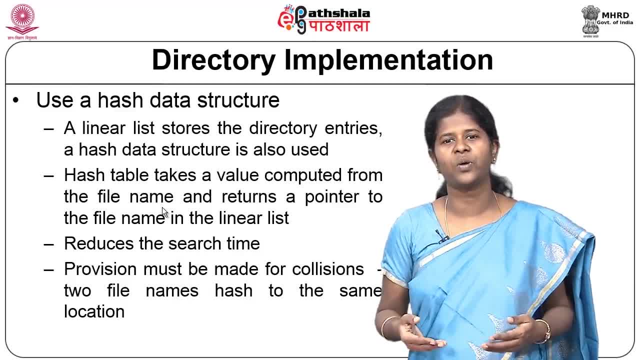 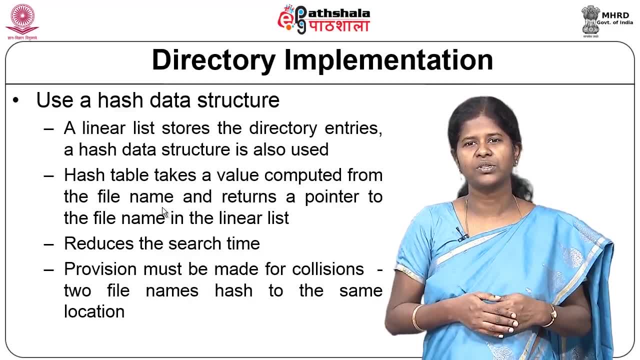 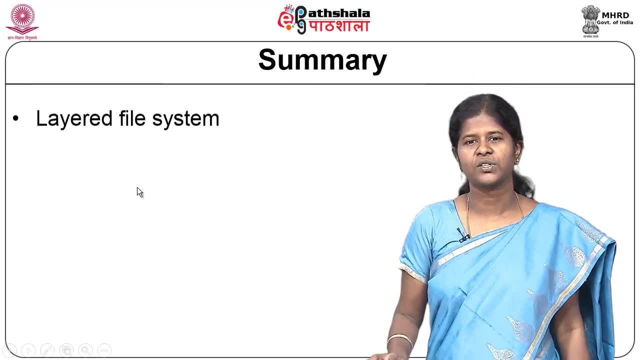 time is reduced, but the problem is that you need to provide provisions for collisions, that is, if two file names they hash to the same location, then what to do So you can have a linear list or a hash data structure for implementing directories. So the summary of what we have learnt in this module is that we learnt what a layered file 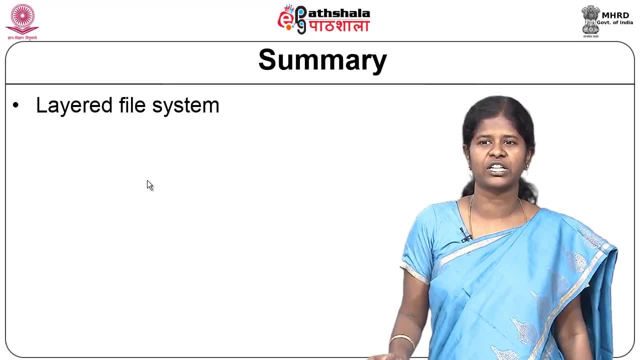 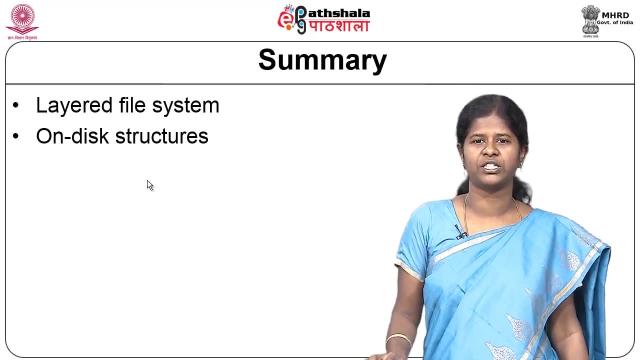 system is. what are the different layers that go to the file system? what are the functionalities of the different layers? Then we understood that a number of on disk structures are maintained to the implementation of this file system and a number of in memory structures are also. 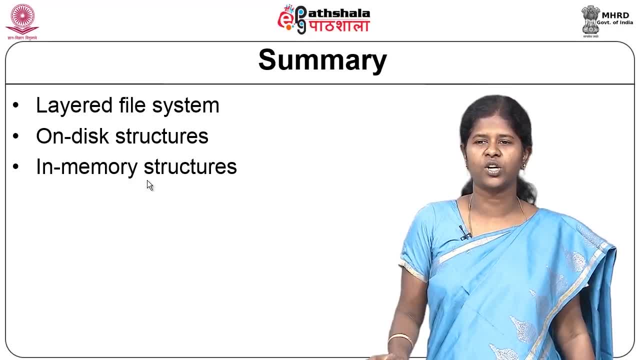 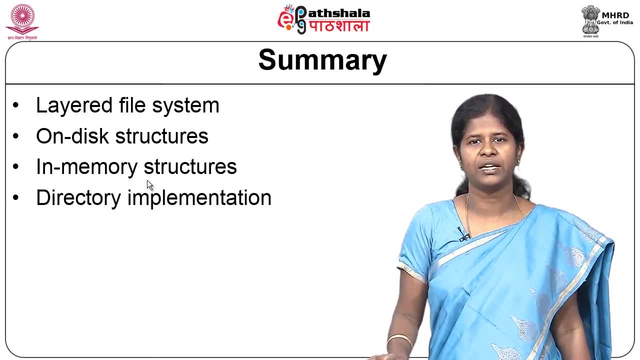 maintained for the implementation of the file system. We saw the functionalities of the different structures and then we saw the different ways in which directory can be implemented: References- thank you. 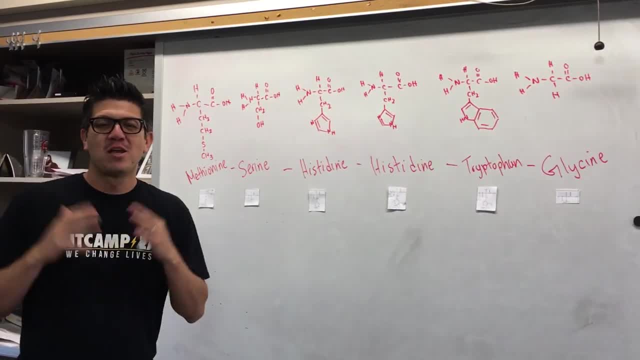 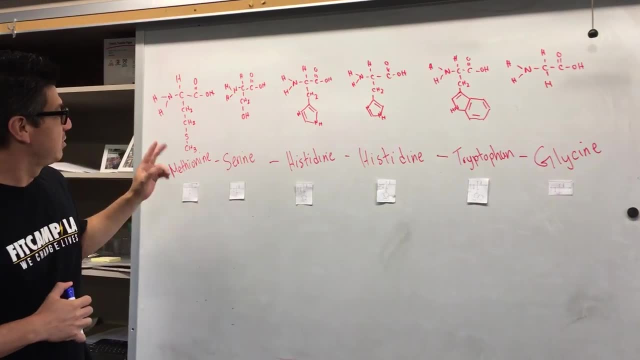 Guys, check it out: MiserBiology360 trying to explain to you guys what a protein is okay. So a protein is made out of amino acids. So right here we have six different amino acids Actually: methionine, serine, histidine, histidine, tryptophan and glycine. right, 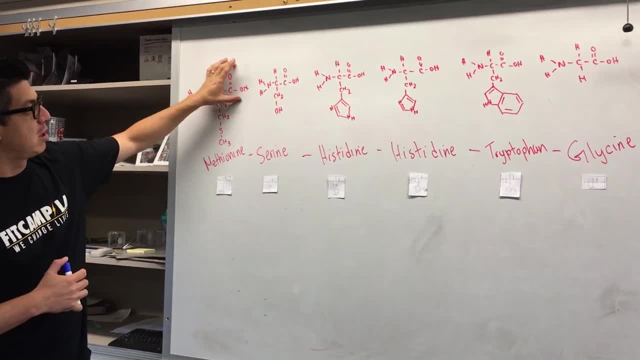 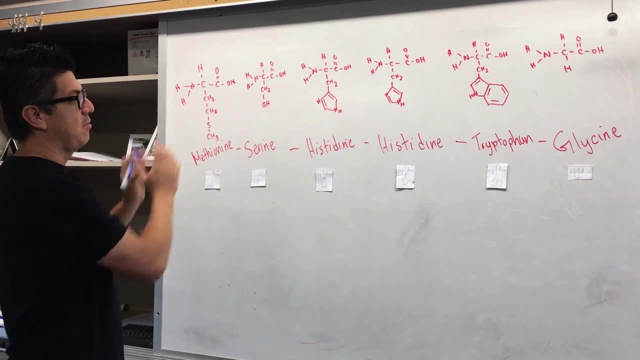 All amino acids have an amino group and a carboxyl group. But in order to make a protein okay, when you're building it, you want to make sure that all the amino groups are on the right, okay, And all the carboxyl groups are on the left, okay. 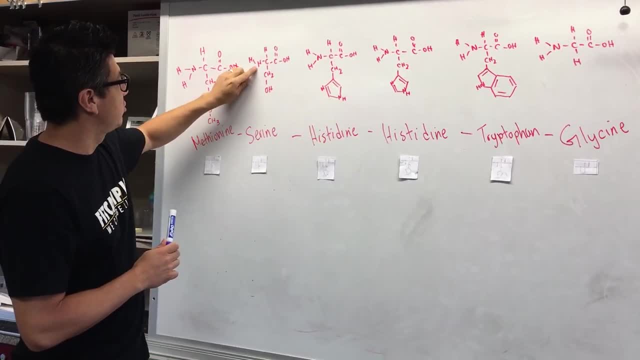 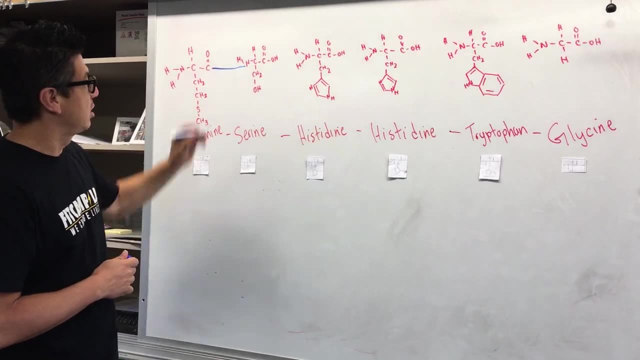 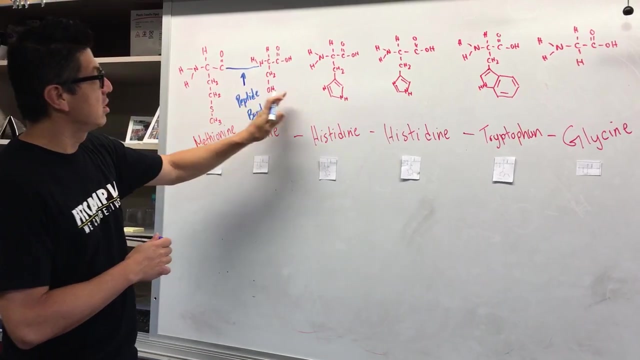 So, to connect them, you're going to take off a hydrogen, You're going to take off an OH, and that's going to let you connect the carbon and the nitrogen, And this right here is called a peptide bond. okay Now, and you're going to do the same thing to connect the rest of the amino acids. 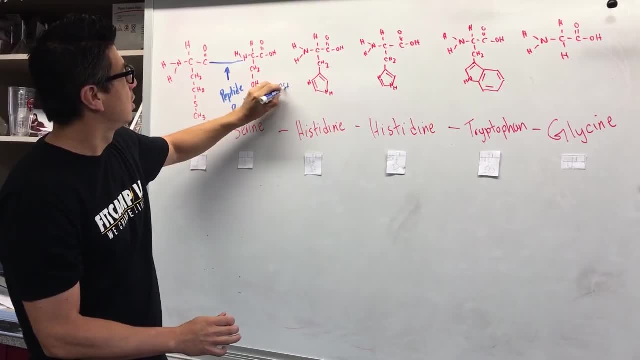 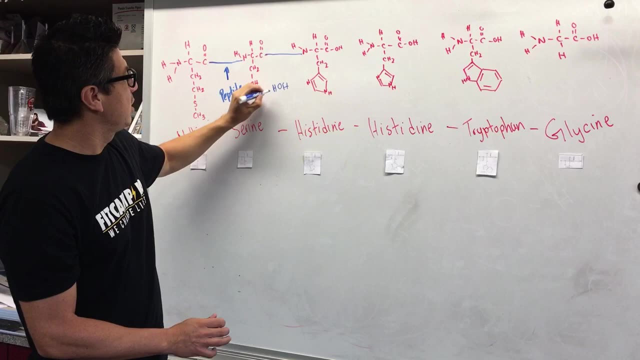 Just remember: The carboxyl loses an OH. okay. The amino group loses a hydrogen. Hydrogen allows you to connect those two. okay, to make your water, and you continue this process until you're done with your protein, right? Thank you for watching.